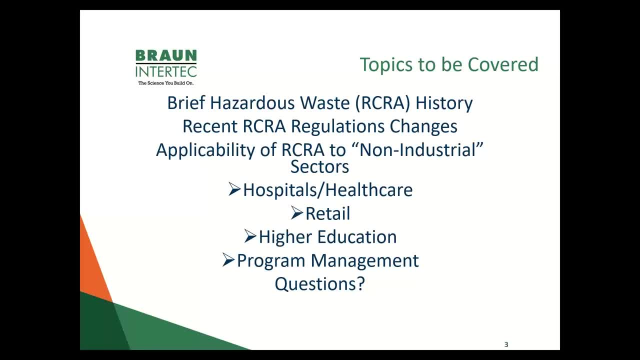 Yeah, And so the federal level regulations in general apply to the what we call- or you know, would be not traditional industrial sectors, such as retail or hospital or higher education areas. Maybe define industry or industrial sectors as heavy industry and refineries and manufacturers and things. 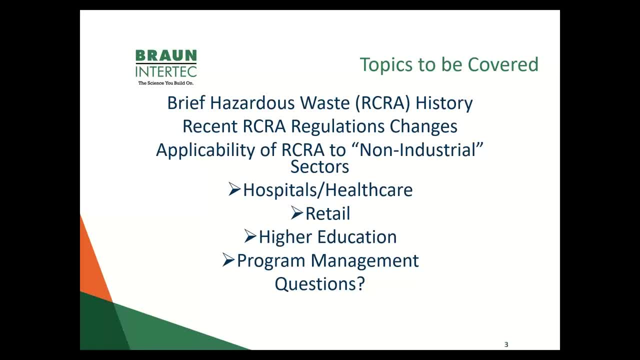 So you know, regulations on RCRA and all the upcoming changes obviously apply to any generator of hazardous waste And and these sectors- the hospital, healthcare, retail and higher ed- our business is just like the rest of those generators, so they have to comply. 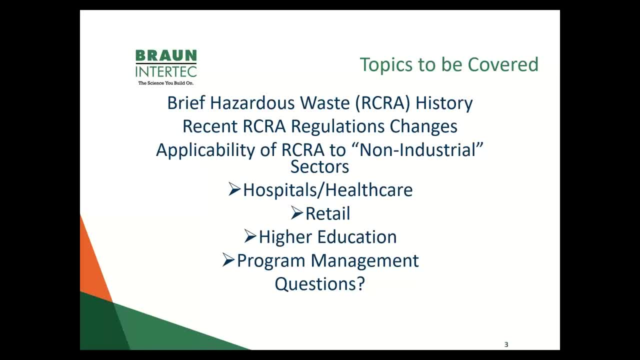 and then at the end kind of, we'll talk a little bit about some program management, you know, suggestions and ideas and sort of the lay of the land and that kind of the enforcement and regulatory climate as it is, you know, throughout the country and in some states today. and throughout this we'll 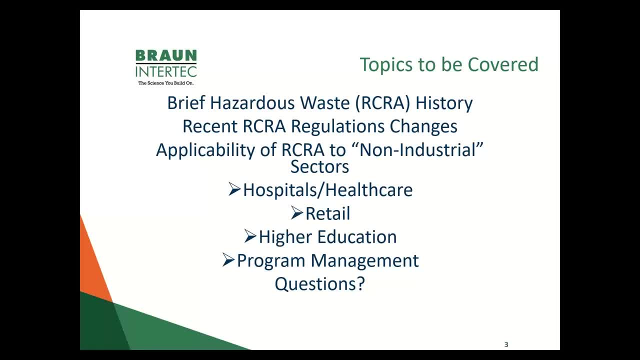 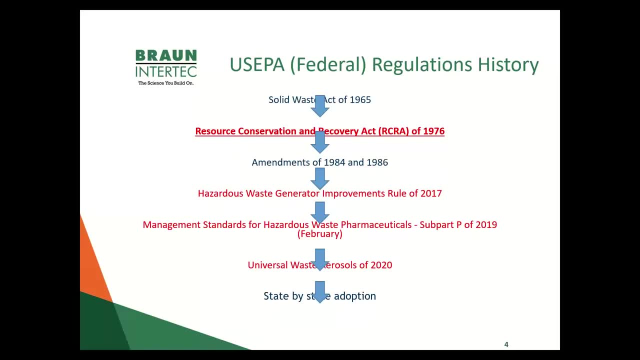 have some examples of some things and should be fun. Oh, got a lot to cover, so so we'll start with. you know more of the. you know the basics on the federal regulations, and it all started sort of in the 1960s of the Solid Waste Act and 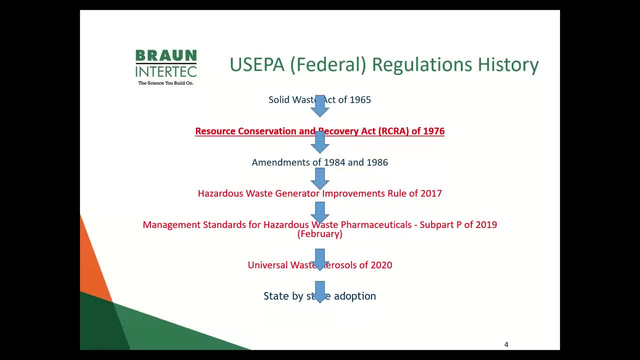 which translated over to the hazardous waste rules, which are the Resource Conservation Recovery Act. so that was came out in 1976 from the federal government. it's been amended a few times, and most recently in 2017, 2019 and then recently in February of 2020 with these: 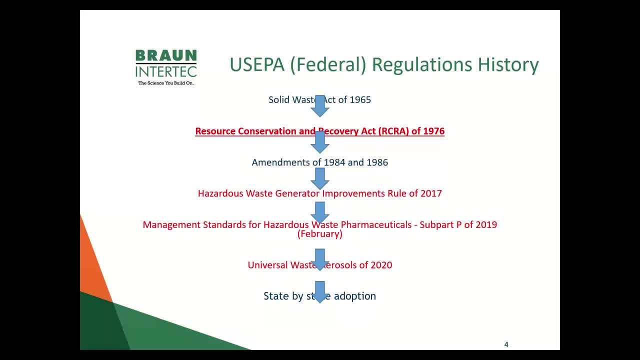 these particular ones and we'll cover these in, you know, in throughout the slides here as well, as you know. then the states have to go, or some states or most states have to adopt or change the regulations to comply with the federal regulations, and then we'll cover those as well. so that's sort of like the 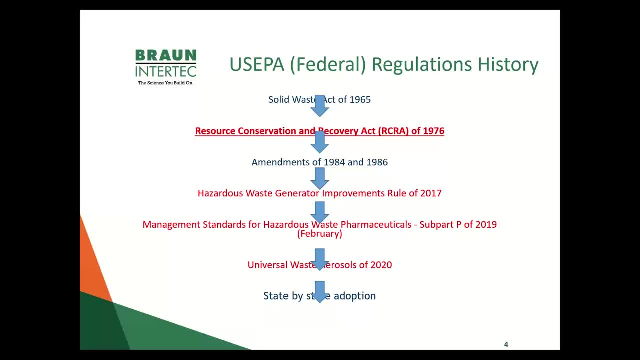 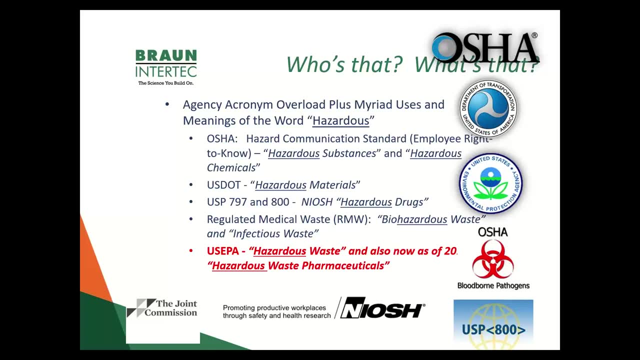 history of what we're covering in terms of the hazardous waste rules and regulations, which all fall under RECRA. well, so what I've seen this is sort of a slide, probably more applicable to the hospital and healthcare industry, but it applies to parts of the retail and 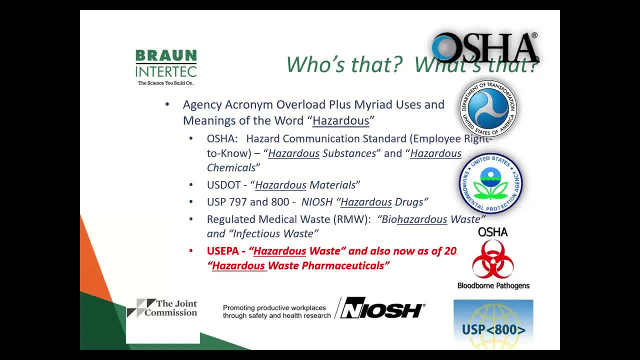 actually part of the, the higher ed institutions that have medical facilities, and really it's just kind of. this was part of this slide came from a friend of mine who is the facility director for, I think, five to six hospitals in the Minneapolis-St Paul area and she's a regional director and 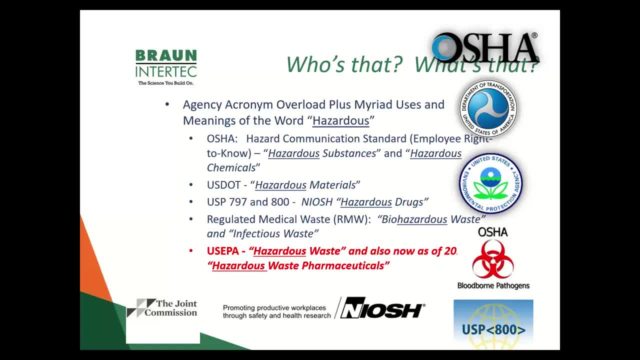 she's. she just uses the word: who is that? what is that? and it essentially the slide is: it's an acronym overload before these generated regulated entities. we like our acronyms a lot of three and four letter yeah, organizations. it's an OMG situation, that's for sure. lol, yellow. that's why I'm here for yep and part of. this is the word, hazardous has and a why. yeah, I mean, and a part of this is the I'd say: if you only knew residents there are, because they actually do it in the territory, they really won't catch those soon. you just give them some minutes, you. 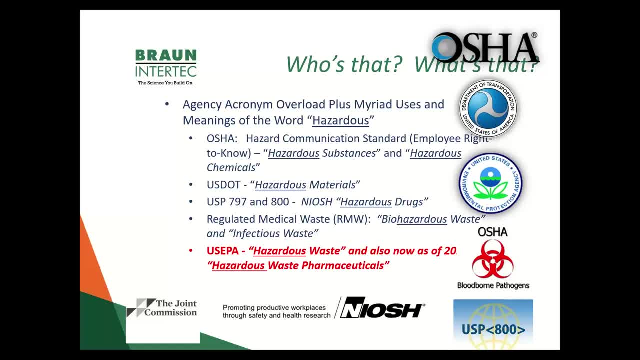 a lot of different meanings in the regulatory world in employee health and safety for OSHA, HAZCOM, Hazardous Communication Standard. Then the US Department of Transportation regulates the world of hazardous materials and they define what that is and how it applies in. 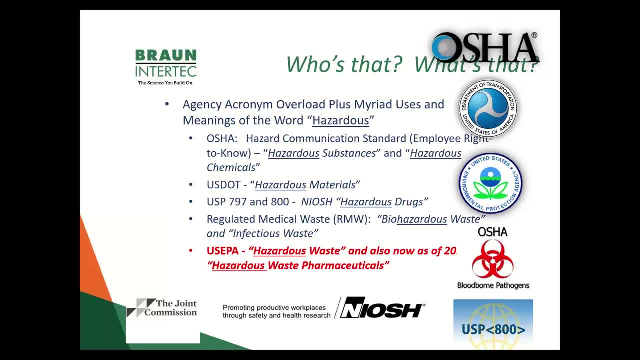 the regulations surrounding that. Then in the pharmacy and the hospital world you have NIOSH. hazardous drugs are referenced in USP 797 and 800, which is something that healthcare and pharmaceutical industries is dealing with, And then we can't leave out biohazardous waste or 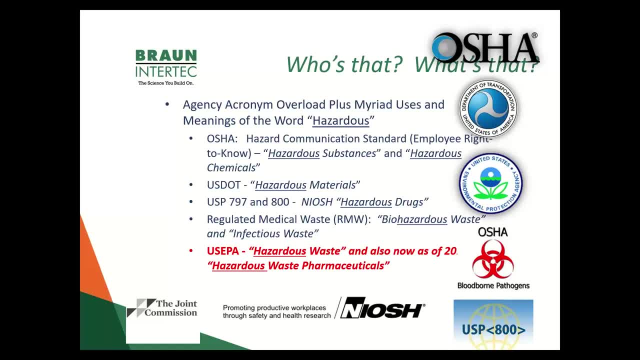 infectious waste. So I would kind of lump those together as regulated medical waste. And the main point is here we get to the bottom. the word hazardous waste and the words hazardous waste pharmaceuticals are distinct And different from the other terms and definitions above And in essence 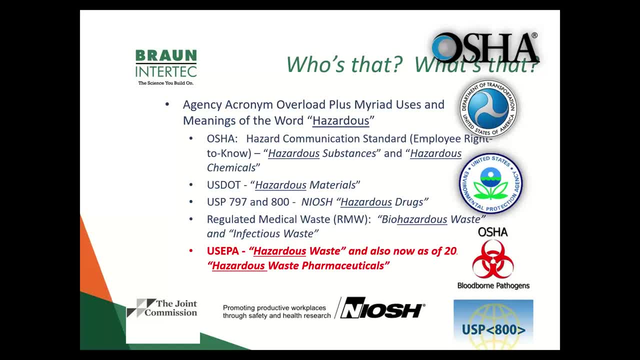 you have to really manage these regulatory areas independently And it's really kind of a challenge, especially I found in the hospital or the healthcare world is. you know a lot of individuals and professionals in labs and nursing and pharmacy. they just think everything is a medical waste or it's everything's a biohaz or it's a hazmat. 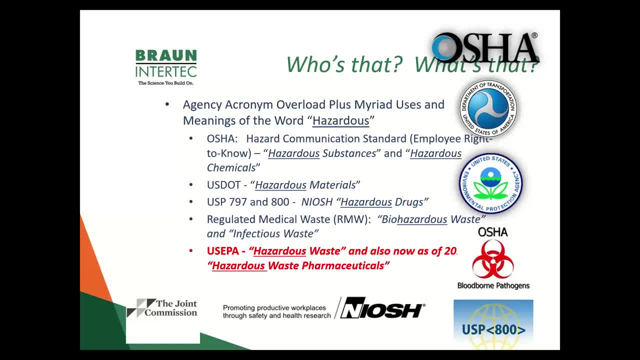 And you really have to kind of pin that down as what actually those are and what regulations apply to those and where they come from, And I think that's much easier, In fact that's. we'll use an example here later on, as I'm helping a hospital in New England states. 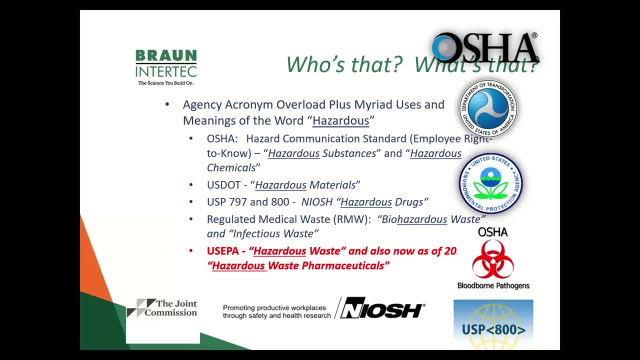 with an inspection right now, and defining these terms and how they should comply and need to comply has been a challenge, because they're kind of stuck in the world of hazmats or biohaz And that's what they know. Dr Andy Roark, You had me. 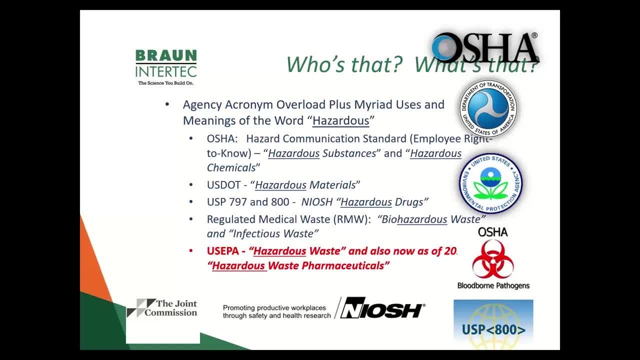 mention earlier about that, things that might have been a little different since COVID. Has that changed a lot? or I mean, Dr Andy Roark, Yeah, it has. You know, in the hospital world, obviously thinking even for the retail business as well, that's consumed a lot of time and resources. There's a lot of activities. 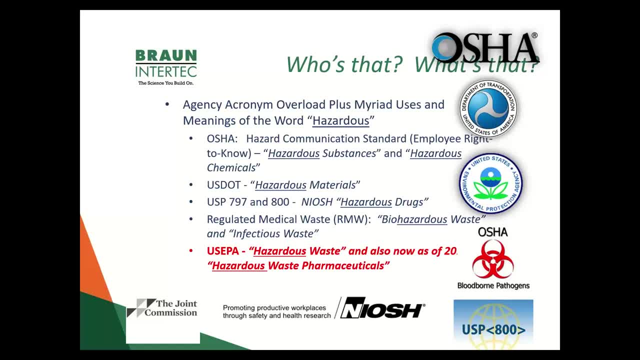 extra cleaning and monitoring, medical monitoring. you know which patients they can have, what kind of waste is generated. Dr Andy Roark, I think to some extent it's kind of settled down in terms of the waste world, I think when it first came about. 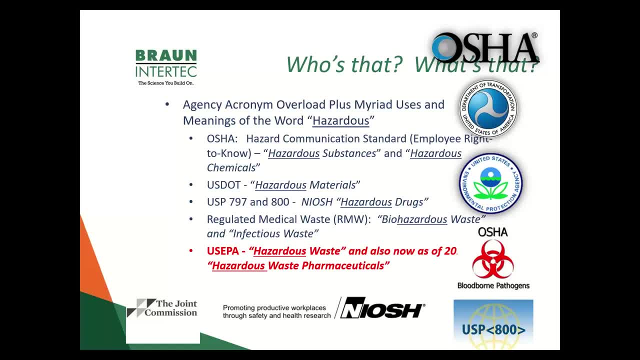 everybody was thinking Ebola too right. So everything is an Ebola type waste And in fact, from what I know- and I'm not a bioinfectious control expert- the COVID waste is kind of what we consider regular regulated medical waste. It can be. 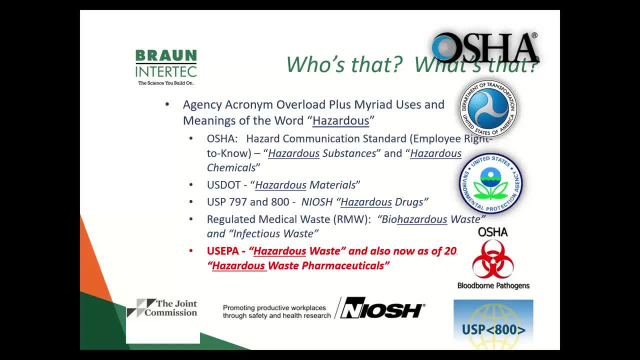 managed in the current practices. Now, obviously there's some extra cleaning occurring, But it's not Ebola, Dr Andy Roark. Dr Andy Roark. So that has kind of settled down, Dr Andy Roark. That's a good thing too. 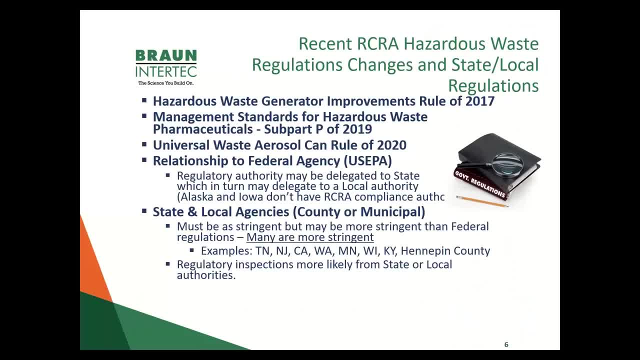 Dr Andy Roark. So, moving on towards these major regulation changes, for RCRA, hazardous waste generator improvements rule is again in 2017.. I'll talk about that in a little bit. Subpart P is the pharma rule and then universal waste aerosol can rule. The thing to understand again, and this is, I think, 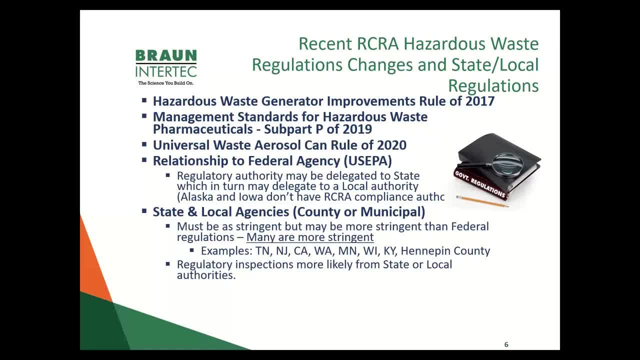 we've covered this before- is the relationship between the federal government- EPA- and the state government, Dr Andy Roark. Is that, Dr Andy Roark? Yeah, Dr Andy Roark, Most states, except for Alaska and Iowa, have regulated authority. So Texas, for example, has the TCEQ, the. 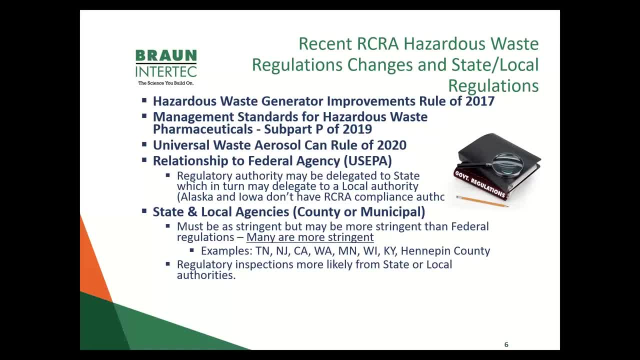 authorized agency in the state of Texas And in Minnesota we have that too. State and local agencies can be more strict, and often are- probably most of them are- than the federal regulations, And I use some examples here, And I think we used this last year because in the Minneapolis-St Paul area. you have the MPF. you know the. that's your legal agency and you're not going to use that in your state. You're going to have to start there. So you're going to have to have a real legislative authority and you might be able to bring this up in the federal regulation. 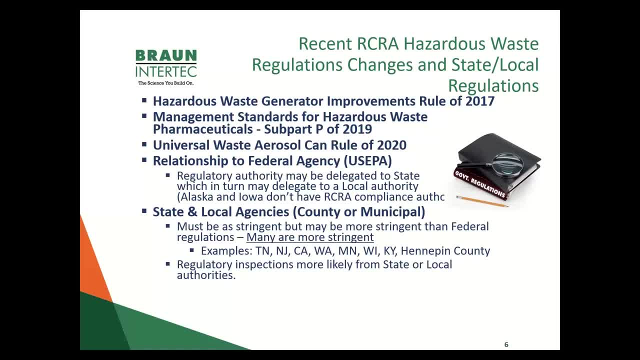 the MPCA, the Minnesota Pollution Control Agency, is the regulated, is the authority, their local 30. but the counties in the Minneapolis st Paul area all have their own hazardous waste program and inspectors. so you know like who would come out and inspect a hospital or a manufacturer or any kind of generator in. 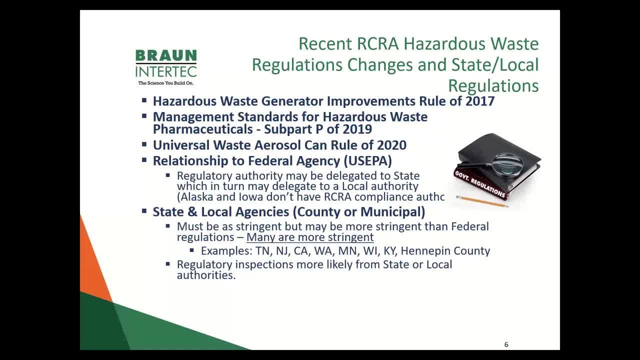 Hennepin County, for example, which is where Minneapolis is located, would be most generally would be a local Hennepin County inspector, not the state inspector. they would maybe go to different sites and then rarely are the federal inspectors in Minnesota. if you're in Iowa, which is just you know. 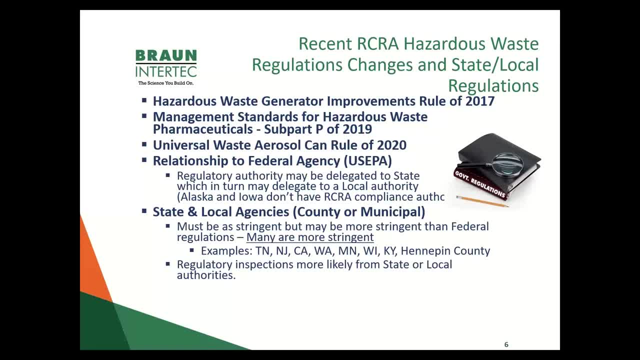 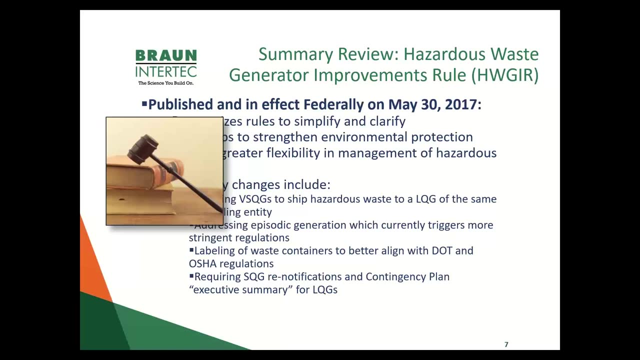 right next door, you would never have a county or a state inspector for hazardous waste. they don't have any programs. it would be a federal inspection gotcha, and in Texas would also obviously be the TCEQ. yeah, I want to make a side note here. I change the format of the slides right before we started, so just to let you. 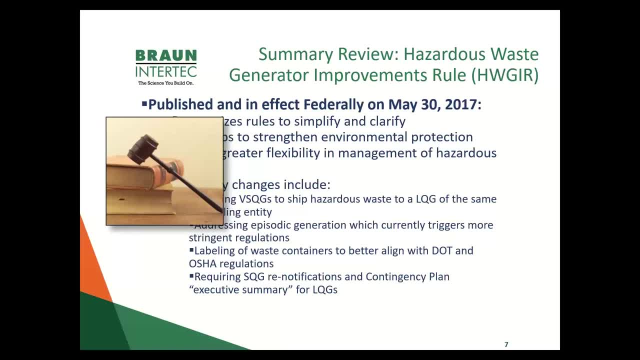 guys know is that I'll be cleaning up these slides. so when you, when you can download them, they won't be. I didn't, I was just noticing the slides is in the picture, so I apologize. all right, that's alright, and none of this is proprietary information, so we'll clean it up. so the the hazardous waste generator. 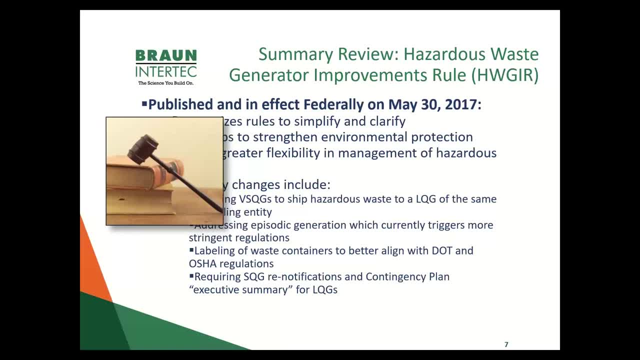 improvements rule again came out in 2017. it fixed a few things in terms of McLaren and simplification, provided some greater flexibility in management of hazardous waste, And one of those was the you know, for example, if you're a, let's say, a small retail organization. 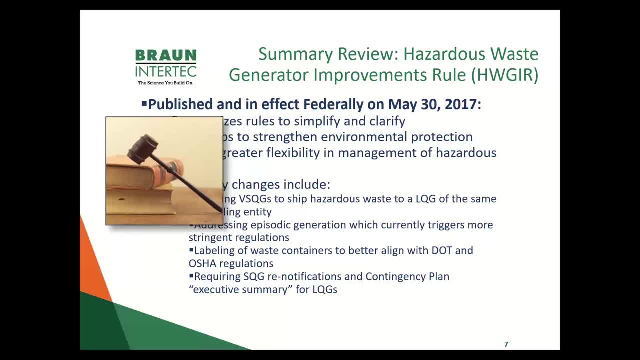 with 10 locations and one headquarters or distribution center, you could theoretically, if all your smaller locations are very small quantity generators, you could ship hazardous waste from those to the large quantity generator or to a bigger facility. It also addressed episodic generation. 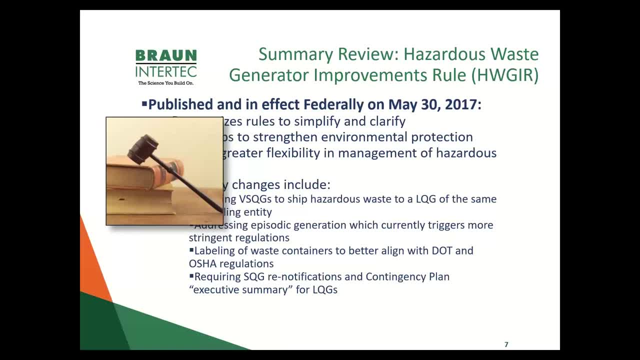 which sometimes had triggered a jumping of one like from a small to a large, if they had, like a spill, or they had a clean out or some activity occurred that put them over the limits for that month, And a few other things which, again, 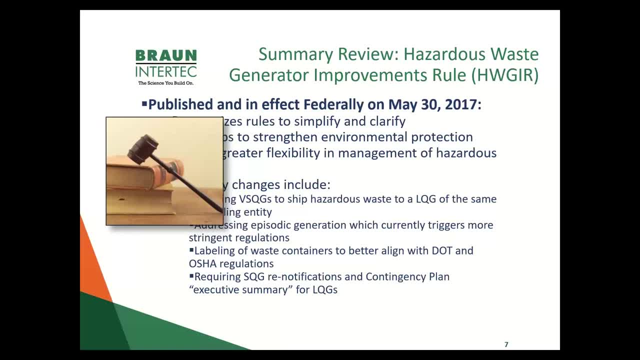 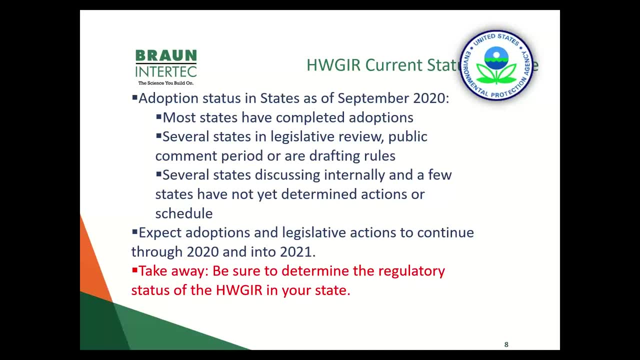 there's more to this than what we have on the slides and what we're covering, So this is for some of the basics. So where are we at with the current status of this? Essentially, as of this month, this is never. 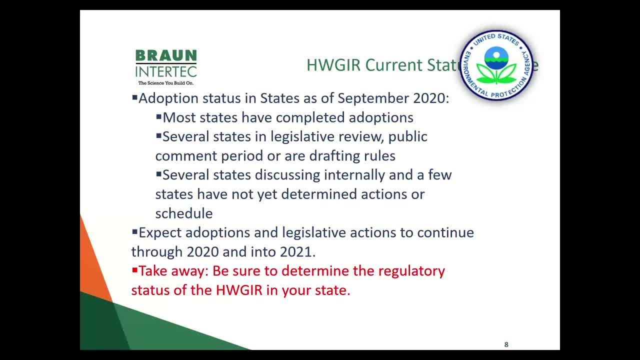 this is kind of a moving target, So it's always changing. Most states have completed adoptions of the hazardous waste generator improvements rules. Some states, several states, are in a legislative review or a public comment period or are drafting the rules, And then there's a few states. 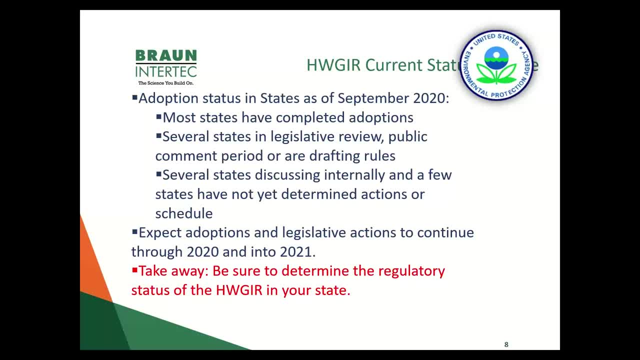 that haven't really determined. they're either discussing internally how they're gonna implement or adopt these, or they haven't indicated anything. you know. no action yet. In a nutshell, it meaning probably we could expect adoptions and legislative actions to continue through this year, as well as into next year. 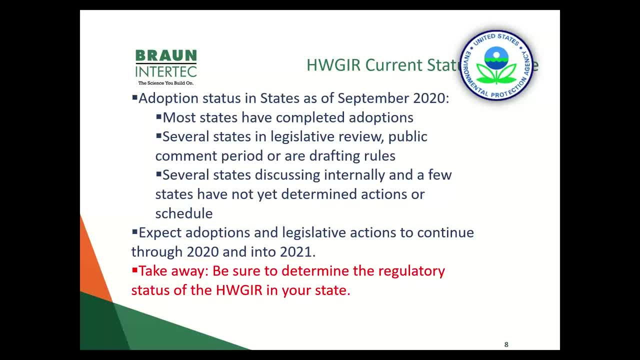 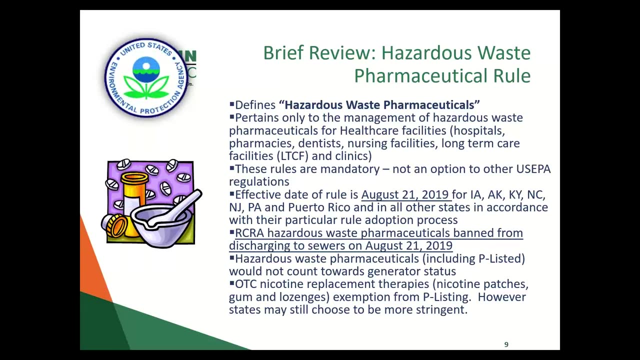 Kind of the takeaway is and all of these, honestly, is to figure out if your location is in, you know, Illinois is to find out where Illinois is with this regulation. okay, The same. we'll cover a little bit on the hazardous pharmaceutical rule. 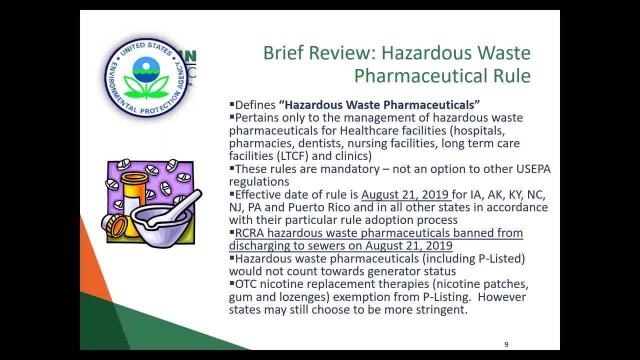 It defines, actually come up with a new term called hazardous waste pharmaceuticals. This regulation pertains to management of hazardous waste pharmaceuticals in what's called healthcare facilities, And I've listed what that's defined. as These rules are mandatory, They're not an option to the other US EPA regulations. 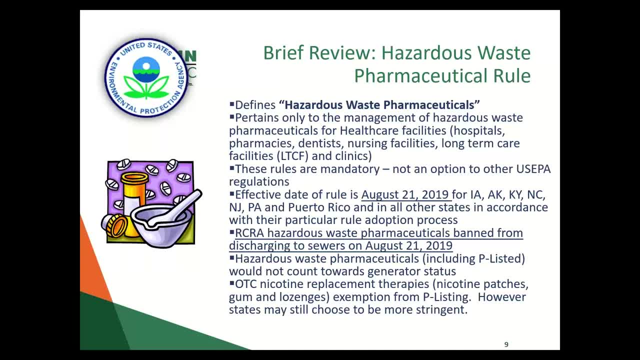 It became effective in August 21st 2019.. And you notice, Iowa and Alaska are in there right away because they again don't have a state program. As soon as a federal rule and regulation is changed, this applies in Iowa and Alaska. 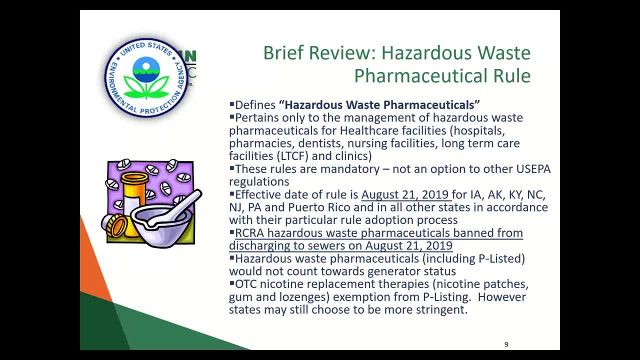 as well as some other states that quickly adopted- or have adoption by rule, Couple of things that maybe I'll go to the second, to the last bullet here, The hazardous waste pharmaceuticals. a key part of this is that if the facility and if the generator is going to manage, 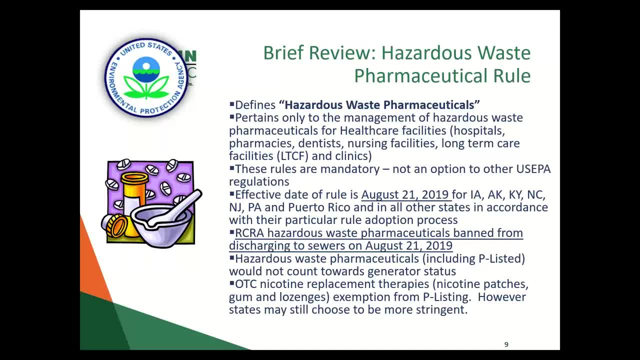 their pharmaceutical waste. in accordance to this regulation, all hazardous waste pharmaceuticals- including, you know, all hazardous waste pharmaceuticals, including, you know, the notorious acutely hazardous P-listed pharmaceuticals- would not count towards the generator status, which is a huge thing. 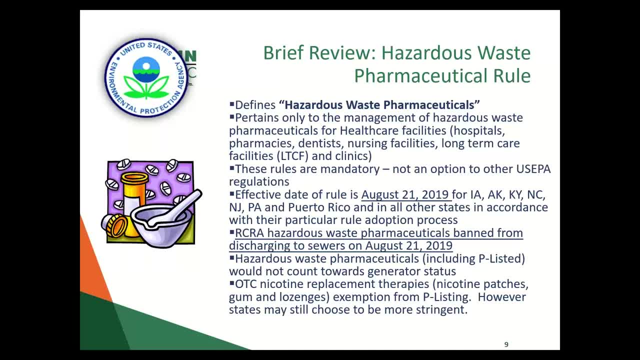 And then there's also was a change added to this as well, kind of a separate thing about over-the-counter nicotine replacement therapies would be exempt from the P-listing. So prior to this, P-075 was the nicotine waste code And for over-the-counter nicotine patches, gum and lozenges 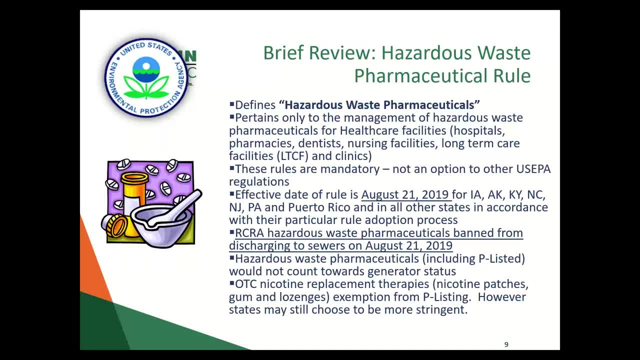 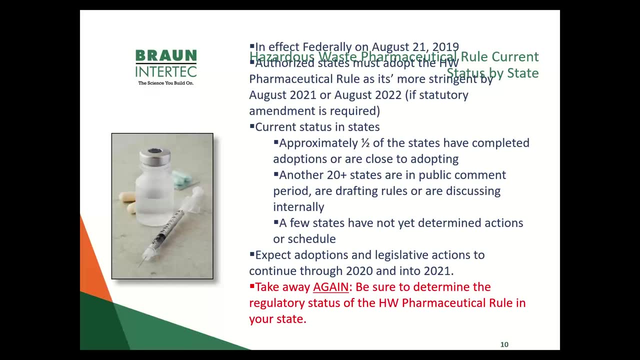 they are now can be exempt. They're now can be exempt from the hazardous waste regulations. The caveat to that is some states may choose to be more stringent on this as they adopt this regulation. Right Again we- I know Lance said he'll move some things around- 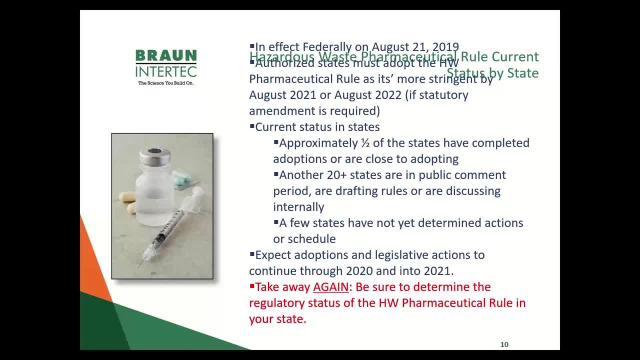 It's. you know, everything's there. So this came in again in 2019.. The authorized states have to move towards the August 2021. august 22 depend upon if they have to do statutory amendments. current status: approximately roughly half of the states have completed adoptions, are very close to adopting, so that's sort of the lay. 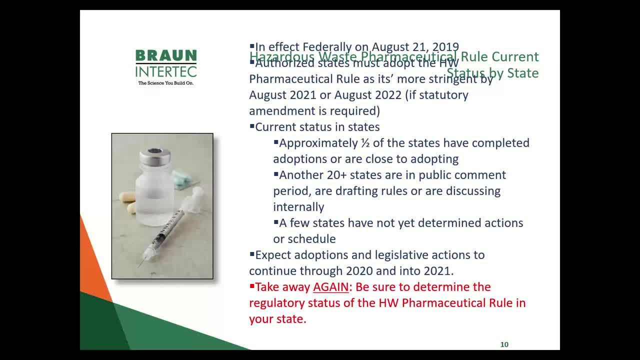 of the land. another 20 are in the kind of the process of doing that, and i think there's a handful of states that have either not decided anything or there's no schedule or haven't really indicated what what their activity is. um kind of a key takeaway again on the bottom, here is: 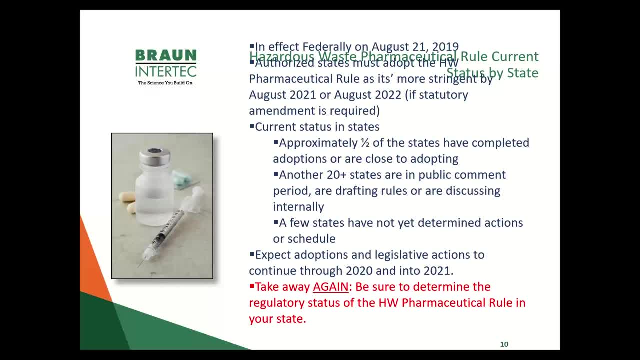 you know, if you are a facility or, let's say, a national pharmacy retailer, you know, is to know what is the status of that particular role in the state or location where you are, and then you can figure out whether how to comply with that. all right. the next one: universal waste aerosol rule. 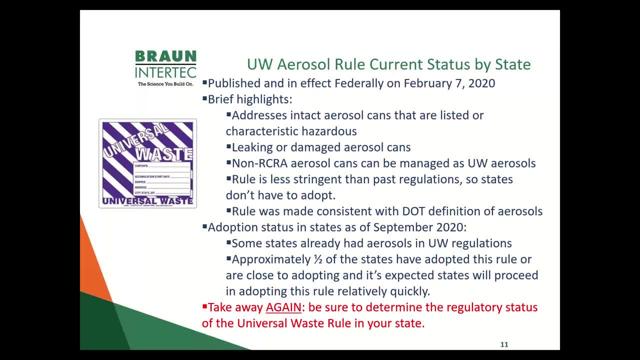 kind of in nutshell. basically, this is intact aerosol cans that are either listed or characteristic hazardous, and it also included a section addressing leaking or damaged aerosol cans. this rule allowed non-rec aerosol cans could be managed as universal waste aerosols too. that would probably make it easier. 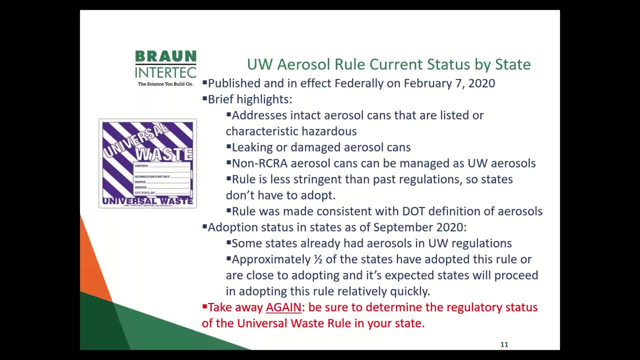 you know, rather than having to determine which is, which, in some cases, is to just you know, manage them all the same way. one of the things about this regulation is the rule is less stringent than past regulations from the federal level, so the states don't have to adopt this. 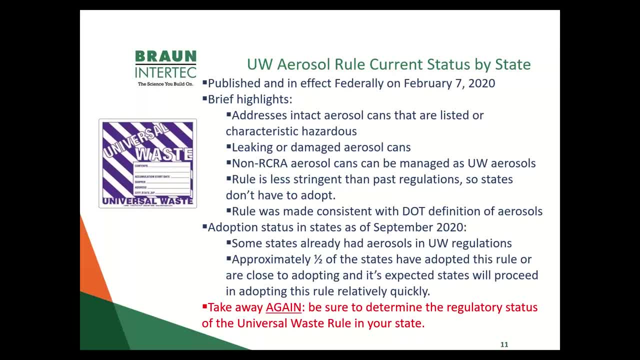 regulation um. so and in some states um eran做 diagonally or electronic regulation um it depends on the state- already had- hes already had aerosols in their existing state universal waste regulations, so it's easy to just um continue the way they were going. and so, again, we think this is going to be moving quick, more quickly than relative to the other, the other ones that are going to take a little more time, which are probably more difficult subject really. so, you know, i try to see if there's a lot of things and at the end of the day too, you can run into this musical Richter regulation. 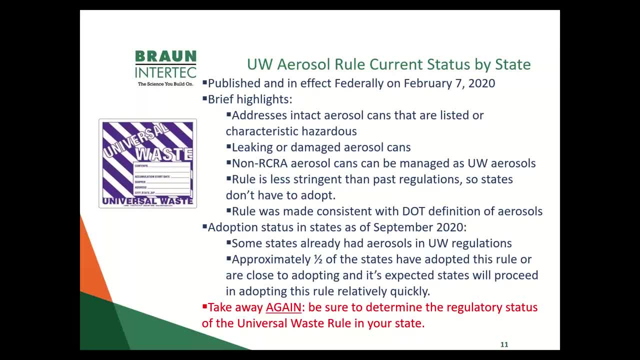 more complicated to some extent, and if you think about what you know where the universal aerosol waste rule would affect in terms of the um, the industries, probably everybody, i mean, who doesn't have these right um, and if you think about the retail industry, if they're especially on the 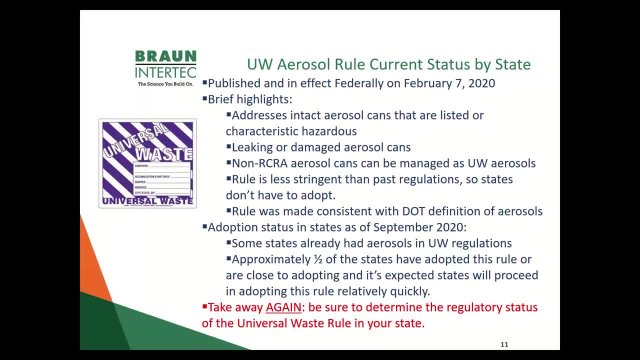 sales side. if they're selling these and it's damaged, just you know this could, this could be this could help reduce their generator status. have you seen like the agencies that are um regulate, regulating this? have you seen kind of like maybe a little bit more of a grace period? 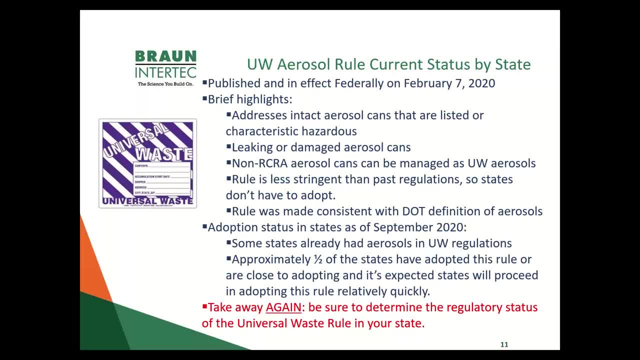 with um, with the covid stuff going on like a bigger fish to fry right now. yeah, yeah, and then in fact that's um, probably that's throwing a little monkey wrench in the timing of individuals because, you know, like a lot of industries, and us included, we maybe were um working remotely. 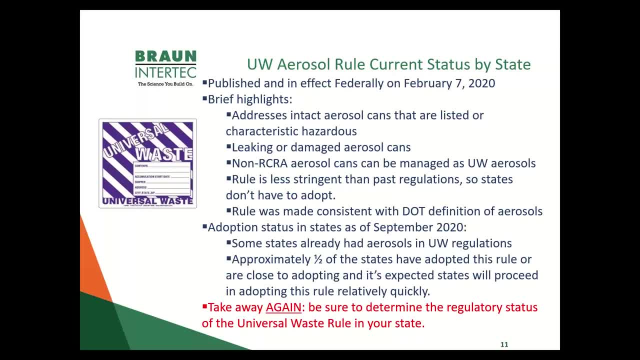 uh, you know, i've i've spoken to regulators who haven't been in their office in six months, yeah, since, yeah, yeah and uh. so you know, things are probably head dragging along a little bit more than than normal. um and and, and, uh, and then in the, you know, obviously in the hospital world, or 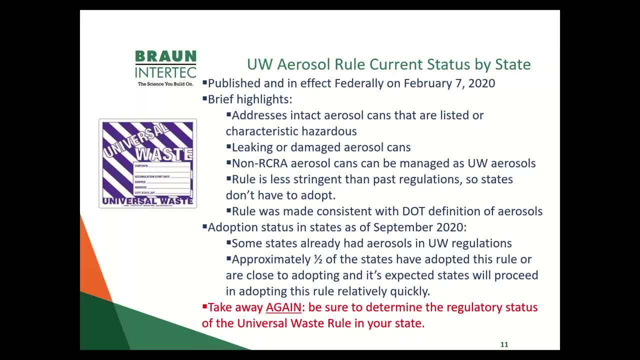 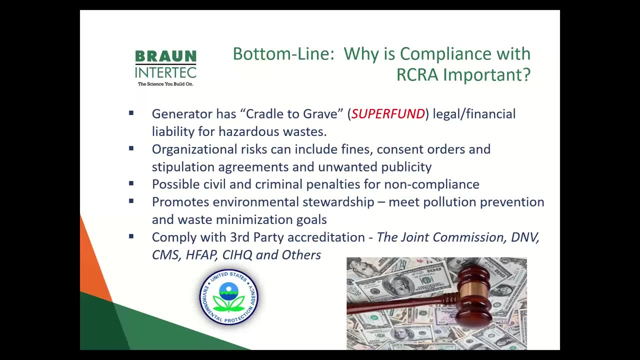 healthcare industry from a you know having the resources that just just to deal with covid in general, other than the regulatory area, um, that's, you know, taking some of their time as well. so you know we come down what would be, you know bottom line what? why is it important to be compliant with the hazardous waste regulations? 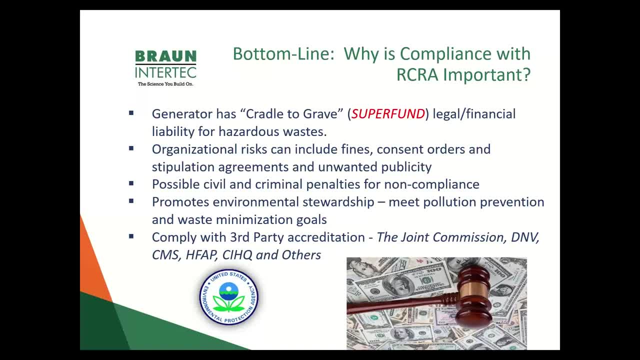 kind of. probably the main thing is the super fund or legal financial liability, because essentially these wastes are always the generators. um cradle the grave means it's generated somewhere and it's destroyed or disposed of some other place, and throughout that whole chain it's, it's- uh, you know it's, it's, it's owned by the, the generator. um, you also have organizational 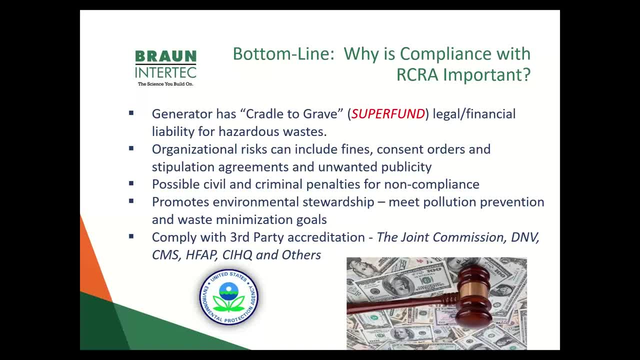 risks, which can include fines at consent orders, stipulations, agreements, you know nov's um, or, in fact, if in the worst cases, it's become some publicity, like you're in the paper that you know xyz hospital, which is, you know, that's not a good way to find out right away. yeah, yeah, in in. 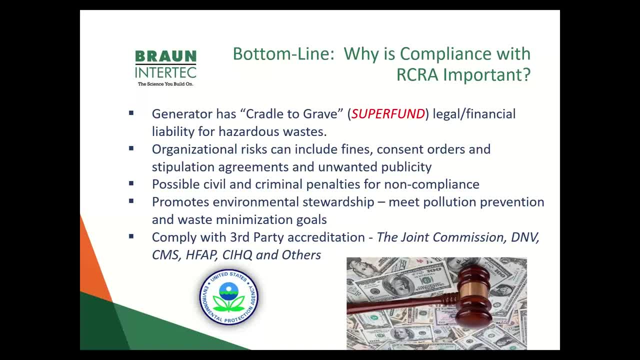 you know. well, you think well, maybe you know they should know what they're doing, or but again, they're going to have inspections. uh, they're, they have a program and there are compliance regulations and requirements and things like that. so it's, it's in their charge to maybe- uh, they don't necessarilyone. 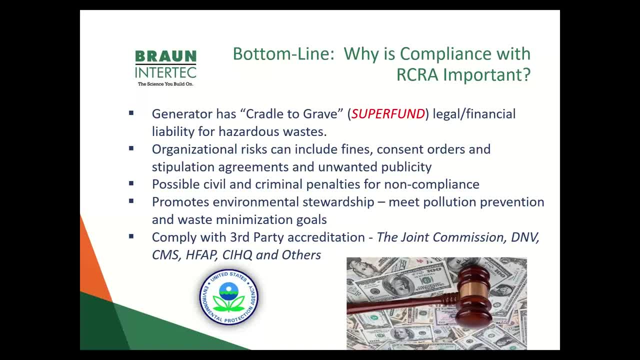 and you have to meet those kind of the bottom line here. on. the last bullet point is in the- especially in the hospital organization or structure or sector, is you have third party or other accreditation compliance organizations that are pretty keen on knowing that you as a business, you as a generator, comply with these regulations. they're not necessarily the agency. 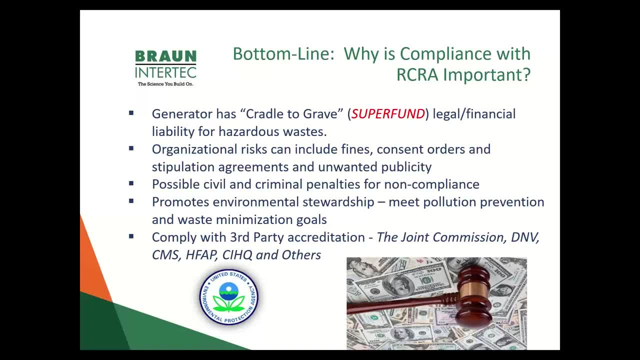 inspectors. they are primarily there. a lot of them are for the centers of medicaid and medicare services funding medical funding, and there's a lot of standards and other requirements that these locations have to comply with so they maintain and don't lose funding from the federal government for 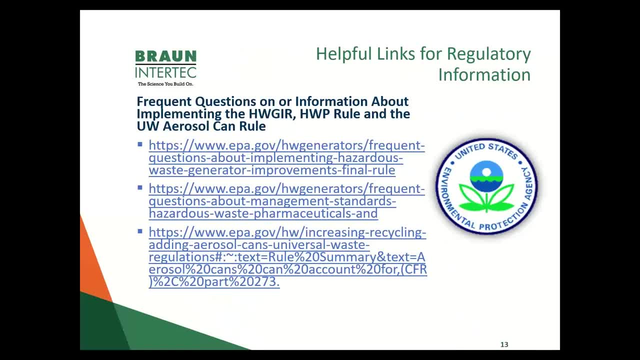 from medicaid, medicare all right, kind of. lastly, and for their updating or regulatory world is where would i turn? and this is these are actually links that i use for questions on any of these regulatory changes. um, one of the one of the i think one of the good things about these- 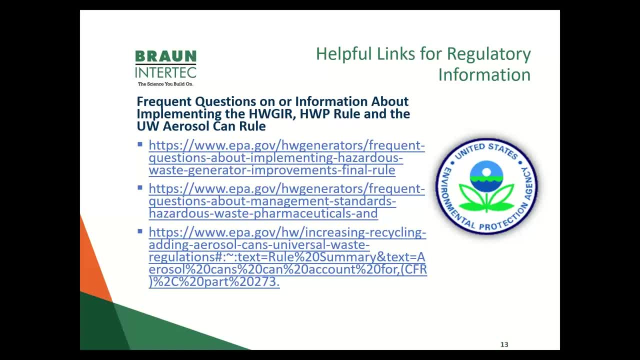 websites is they also. i think most of them, or several of them, have the links to the state agencies as well. so you can literally click on, you know, the federal one and you can scroll down and you will have the various states and it will give a either a summary or a link to that state agency. 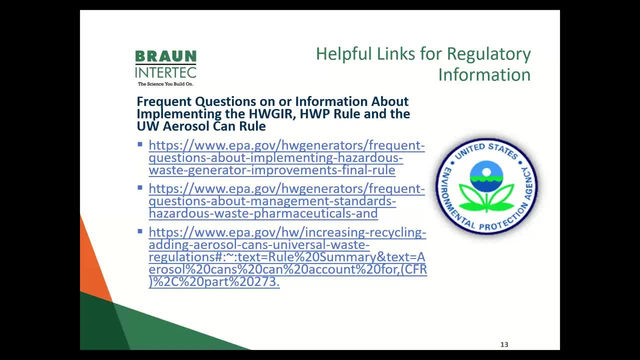 so that you can determine, drill down basically and see what, what is the status of these particular? you know, regulations changes, yeah, and most of them in. you probably already said it. but i was like, even though the epa has them, you need still need to check state and local, obviously, for 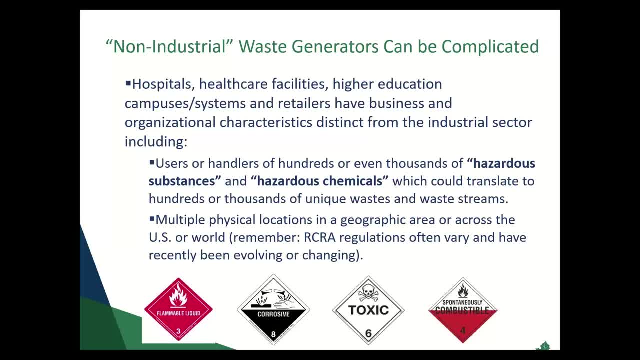 for different changes. yeah, yeah, and um, kind of what we talked about too is there's there's a little drag on updating. you know, some of these changes in the this, for example, you know a state may adopt this and pass it, um, and they, they don't get around to updating their website for a month. 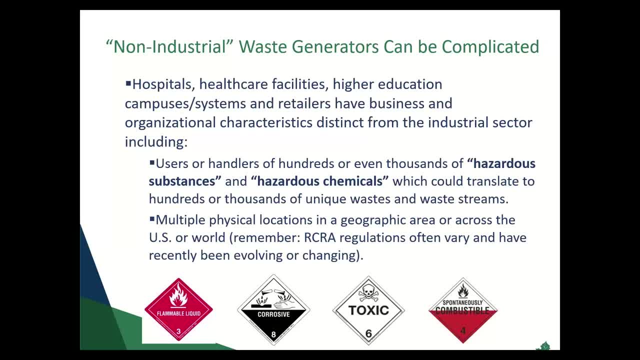 or two or three. so you know, sometimes it's worth a phone call, okay, um. so on to the what we call. you know why? why are we looking at what we call the non-industrial waste generators? well, and in reality they can be as complex as um as the bigger generators. in fact, i, i would say in some cases, or some. 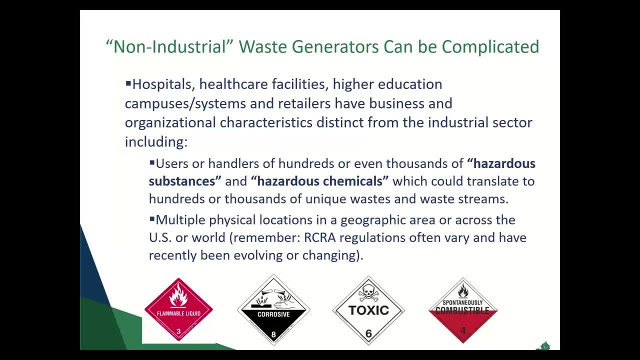 reasons why they are more complex. um, so you know, part of it is the. they're either users or handlers, or they consume or they purchase hundreds or even thousands of hazardous chemicals, and some or many of those can be, uh, wastes that are have to be dealt with, and, um, and if you add in 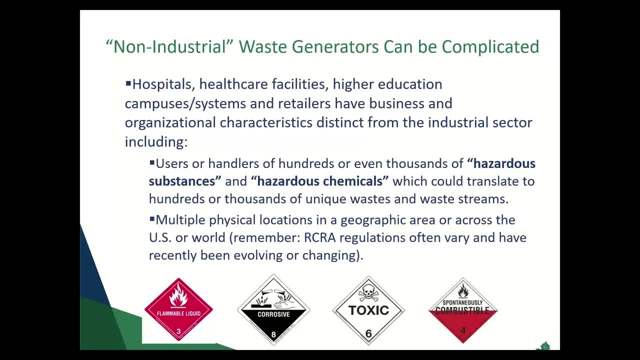 for example, um, um the retail industry, or even there's hospital systems, with- i think i'm working with one that has close to 200 hospitals and another 4 000 off sites, maybe 2 000, wow, remember, um across 15 states. um, and then in the retail world there's obviously there's national retail. 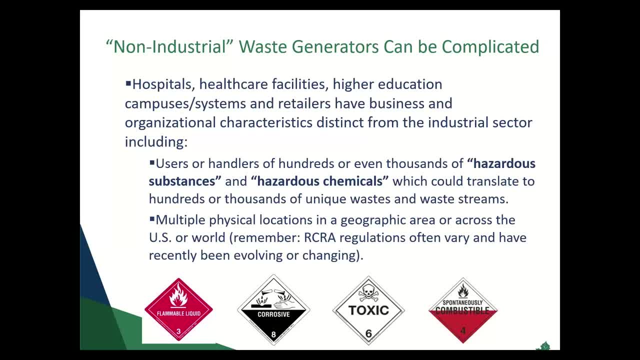 organizations that are in every state, with thousands of locations, um. so mapping where those regulations are and how they're changed and how they're changed is a big part of the process here, but i think it's a great way to understand as well that what you're really. 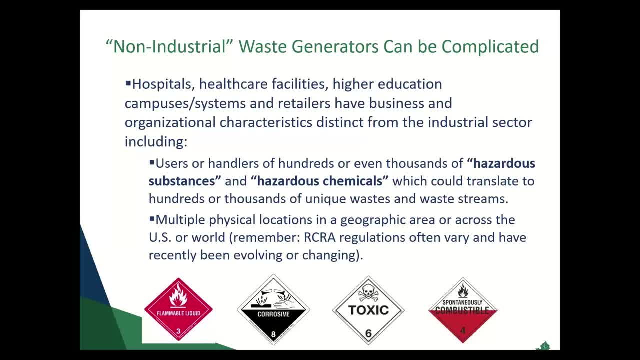 looking at is the number of people that are involved in something that has been a real impact, and to find out what the impact is on the cleaning up of the waste generators and then making sure that it's the right things to do. you know that they're just being. 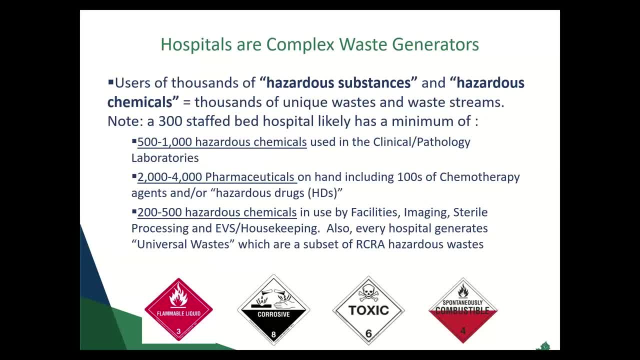 applied to the waste generators. um, i think that's a really good idea. um, i i think that's what, because you know it's. it's true. there's, in fact, a lot of people in the inventory of places like in philadelphia and one of the other places in the country. there's all kinds. 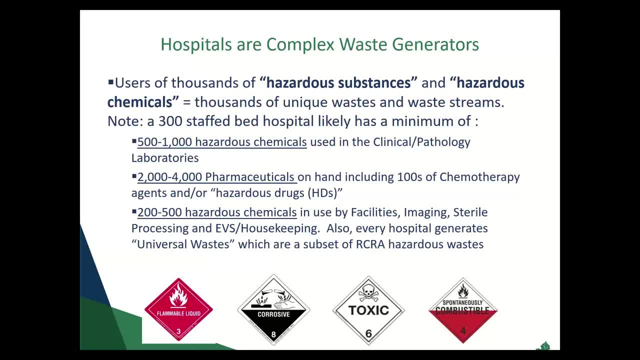 of things that are going on. uh, so that's. i think what i'm finding is that that's, that's hospitals, and it's hard pin this down. how many exact chemicals are in your building? well, these are ballpark ranges and you know, you take a, a Dallas. 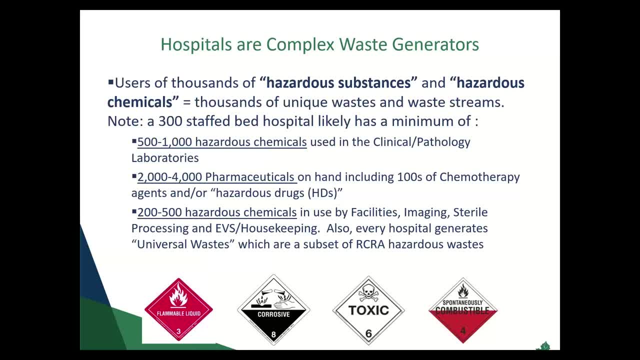 Fort Worth metro area major medical campus might have double or triple the number of these in in the building any given time, and so it's it's very tough to to know what's in your building from a chemical standpoint, and then which of these, and which combination of these, in some cases are the actual waste that are. 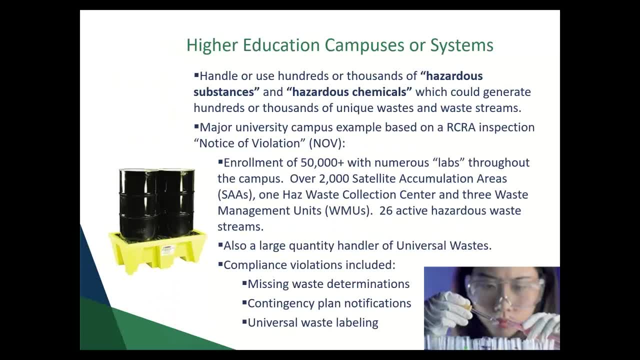 being generated and then if we kind of roll into the higher education campuses and systems and kind of like, look a little bit similar to the hospital campuses in some respects, but they get a handle and use thousands or hundreds of different chemicals. I happen to was looking into inspections. 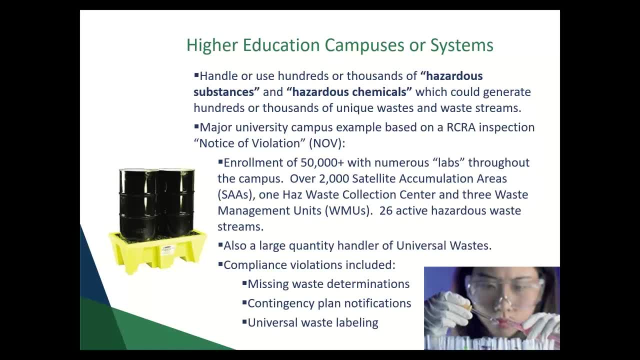 and I was looking at a lot of different chemicals and I was looking at a lot of p? acontecies type of- and though it's a violations- university or higher educational campuses, and I found this one, so I kind of use it as an example here. this particular example is: 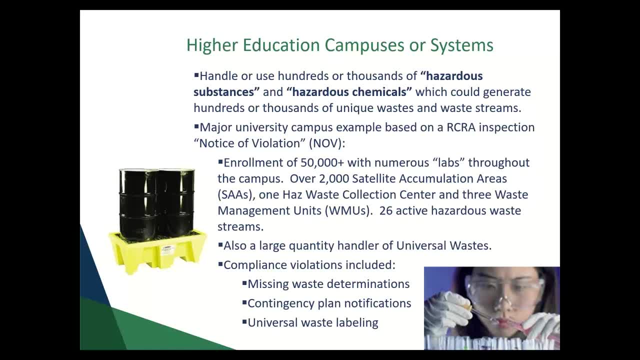 large state university with fifty thousand plus- actually it's quite a bit more than that I saw in Roman, with numerous labs throughout the campus and where hazardous waste is being generated. hmm, I'm just trying to fathom how to keep track of that. um, I would say, in a hospital you might have, let's say, a 300. 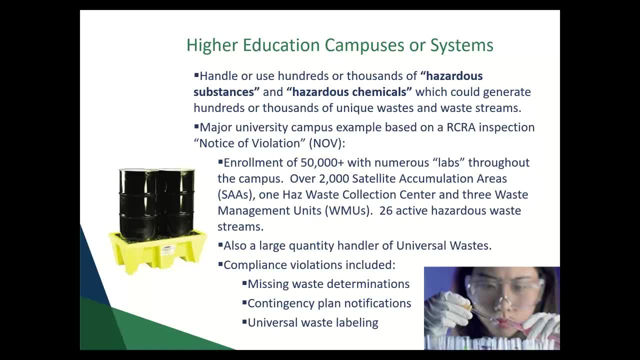 bed hospital you might have 50 to 200 mmm, maybe 50, 200, and hopefully not one person's just responsible for that. so how would one? yeah, how would I would think that that would need a team for sure, yeah, and and then there was. 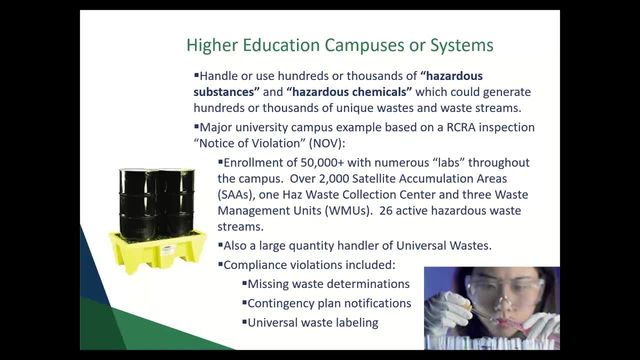 definition. I kind of read the narrative here by about one hazardous waste collection center sort of where all the waste goes, and I know three waste management units and what's interesting is they listed 26 active hazardous waste streams and the. I want to point out that that doesn't necessarily mean twenty six. 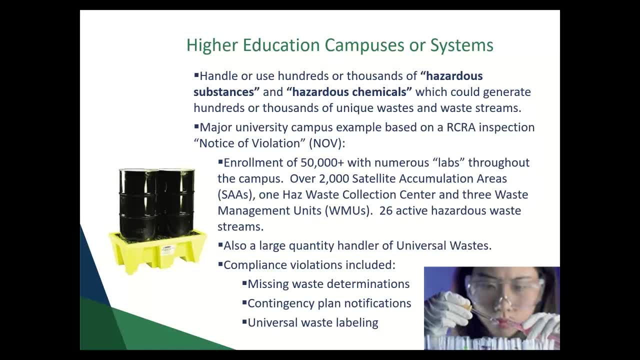 hazardous wastes it could be. some of these waste streams are a lab pack you know, like, for example, flammables d-001. flammable waste from a variety of labs might all come into one location and they put it in a 55 minute place. um the University of Minnesota is doing also on this slide. 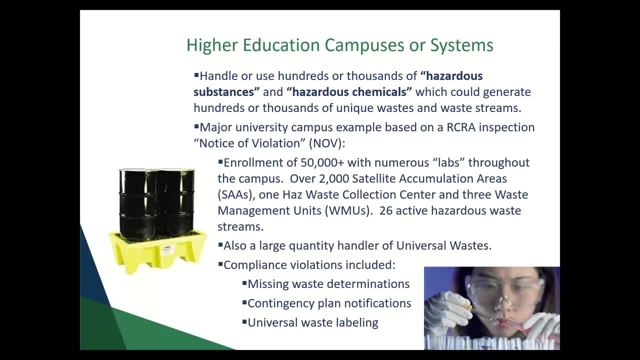 gallon rum and ship it out. that way could be mixing things that are the same can be mixed together. you know all is flammable so that waste stream might be, you know, alcohol, lab waste and it comes from multiple locations. I also noticed that this particular hospital was a large quantity. 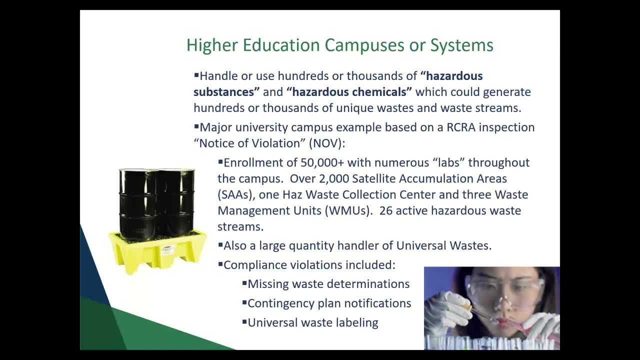 handler of universal wage, which would be the used bulbs and batteries and pesticides and mercury continuing equipment. so that's it's. you have to be a big facility or campus to be a large quantity handler of universal ways. Wow, and and then obviously at that level, then there's some. 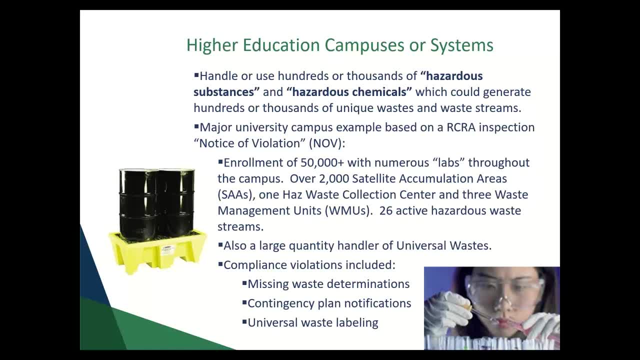 compliance requirements that are attached, that. so really, this could be any. I mean, it could be any college. well, this is, yeah, Texas, actually, or anywhere. yes, this, I think this is a pretty standard description of what you would see at a college campus and you can you know if it's only a 5 000. 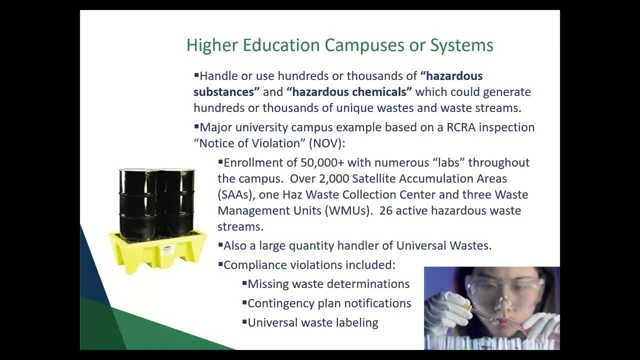 person. you know Community College. it's not going to have anywhere near this right. I mean the large you are in terms of a state college or um research and development, or you know that sort of thing, or the you know you have a- whatever, a niche in the. you know chemistry, or you know um whatever some. 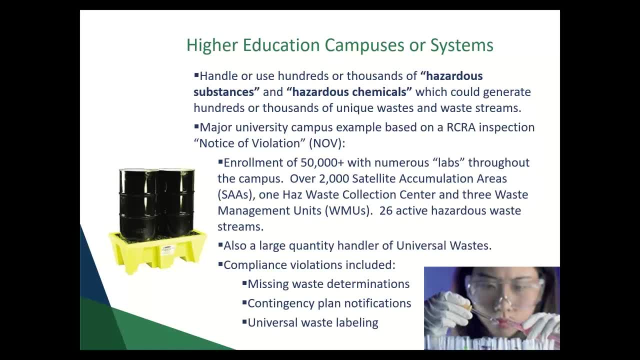 other industry that might have have unique labs, then you know that would apply here. and then again at the bottom here I sort of listed some of the compliance violations. that included missing waste determinations- not really not, not to you know- unexpected type findings for that size of facility and in a in a college like. 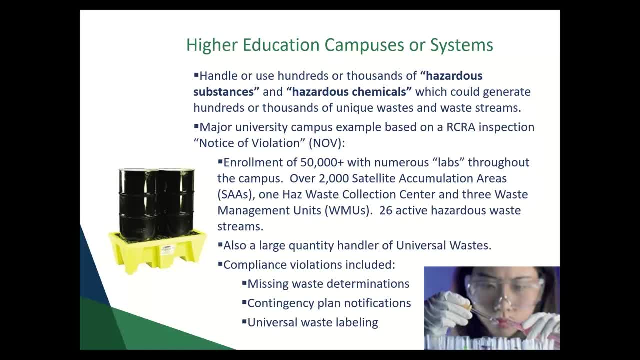 that who would be the ultimate go-to to find the answer guy, like who would be ultimately responsible? well, the uh, the uh in general- and I had this at sort of a wrap at the end- in general, what I've seen in the what I would call the higher educational institutions, like the larger systems, is there. 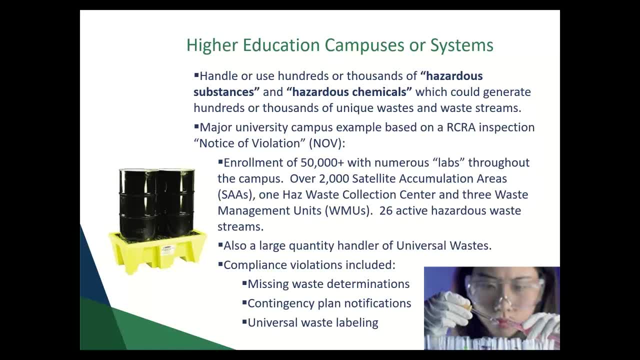 are individuals. there are ehns, environment, health and safety type individuals, or teams or leaders that this is part of their wheelhouse. okay, um, and in fact in some cases they even have. you know technical services, individuals that are has whopper trained, you know they can do lab packs. 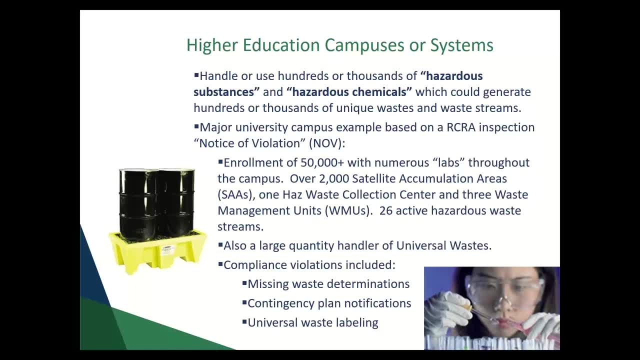 they know how to do manifests. uh, that's what I've seen in that industry, um, I think even to the extent that, uh, educational institutions have run medical centers. I think there's some overlap in that as well. I mean, they're they, they have it's sort of a unique fit at both of these where they have. 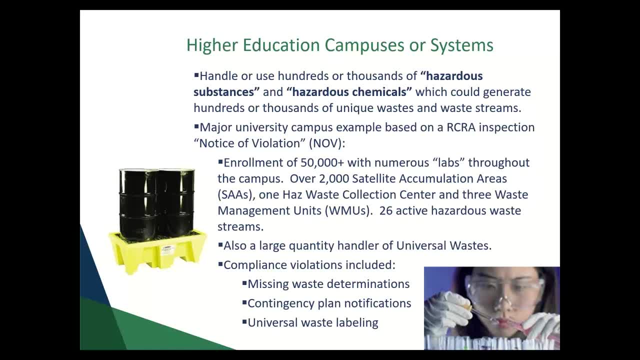 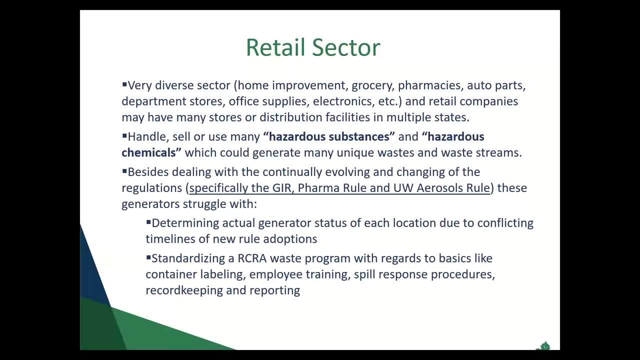 some ehns capability and expertise and and so I think things are pretty well run um. but again they: there's changes and there's, and then you still have to adapt to the new regulations and that may change what you do in a process. so you know, turning more toward the retail sector, you 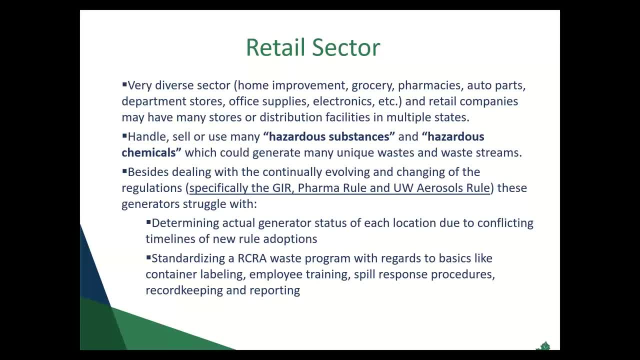 can imagine how this sector is. you know, from one mom and pop type locations to um, you know 5 000 stores. you know home improvement locations, with their hundred and whatever number of distribution centers, um, so what do they do? what do they handle, sell, use? you know a lot. 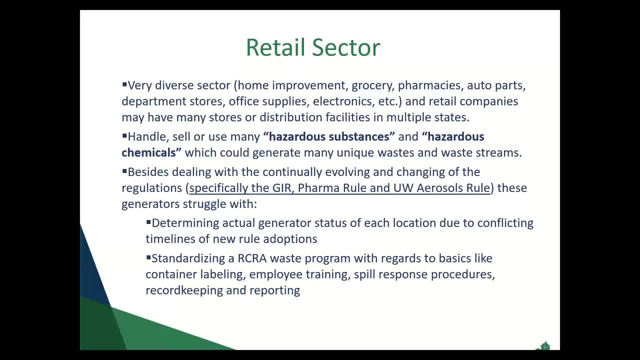 of different hazardous chemicals and you kind of fall into the same. um, you know, pit is that you have these kind of wastes then, because if you can't, if it's damaged or it leaks or it spills you, you can't put it on the shelf and hope Lance French comes up and picks it up. right. 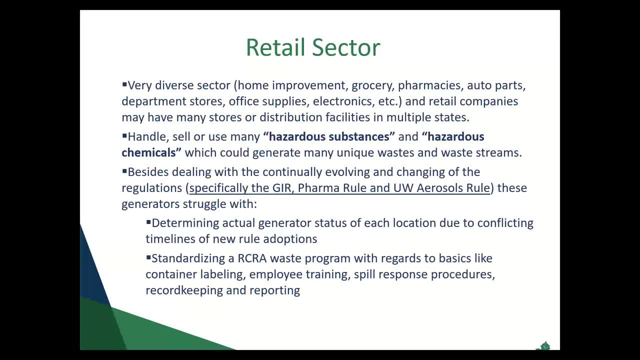 you know you're not going to want it. it's got a dent in it, yeah, and actually, and if it does spill, you need to make sure that the person that is handling the spill knows what they're doing, otherwise they just- I hope so, yeah, because otherwise, you know, you spill some paint and 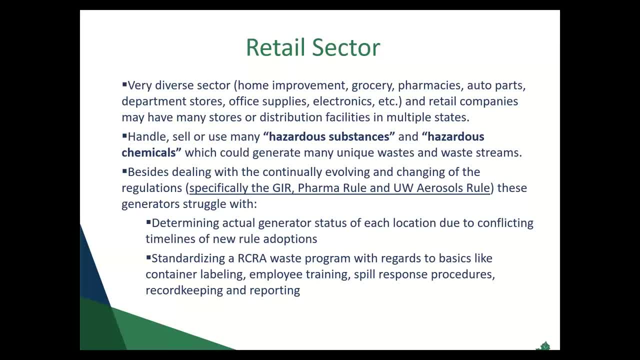 Home Depot and then just put in trash. that's that, you know. that's a you know. I'm sure these places have like entire aisles that are hazardous wastes, if, if they got out, yeah, or spilled well in, um, you know any of the like the paints areas or the? um cleaning products, um, if you're a retailer. 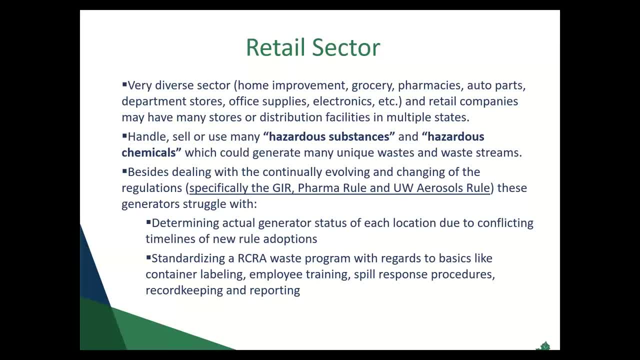 that has a pharmacy. you know, you've got that angle as well. um, there's just, it's just, it's kind of a monster. yeah, there's lots of different things, so the kind of the couple last points here is that when we covered earlier the uh, hazardous waste generator, improvements rule the farmer rule the. 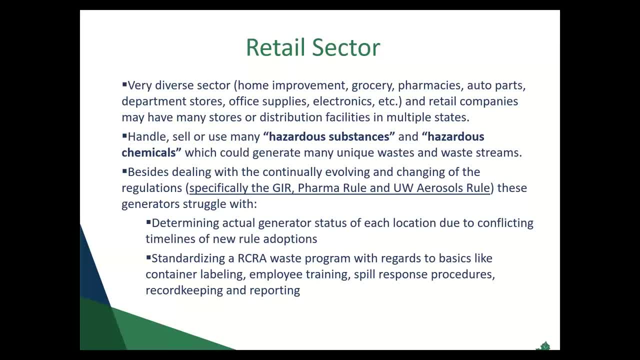 universal waste aerosols rule. all these things are sort of adapting and changing throughout the year at different schedules. if I'm a retailer with 5 000 locations, how am I keeping track of my generator status? because all of those could change. the adoption of those regulations could change. 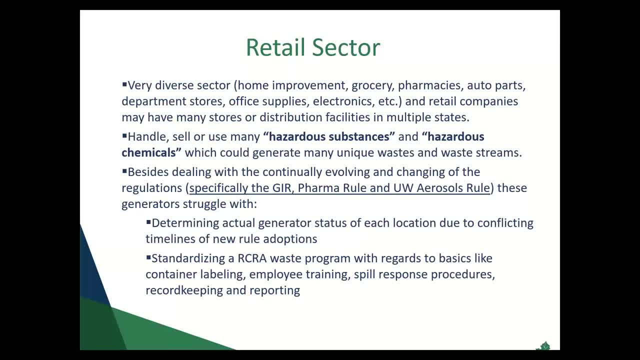 what I'm actually doing. um, and then standards: standardizing a program, which ideally that's what you'd like to do. you know, if you're, if you're one retail location in one state it's, then that's pretty easy to figure out what you're doing. if you have to now figure out for 50 locations, 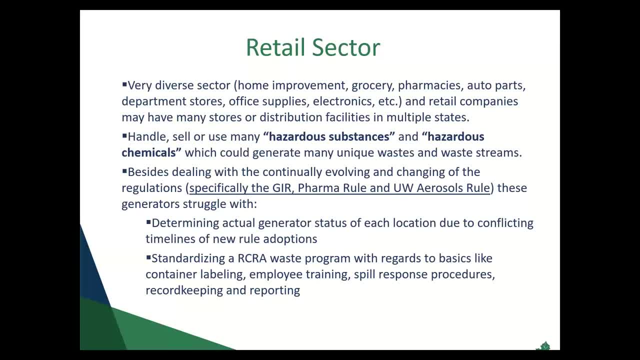 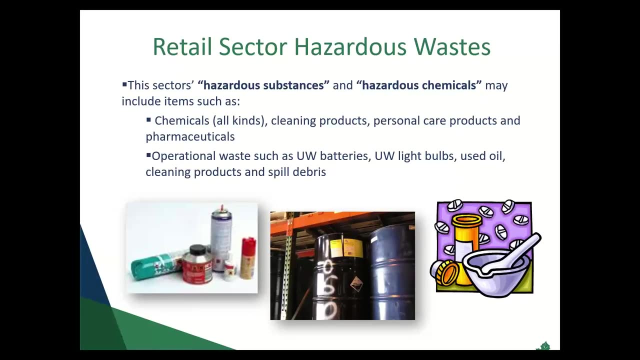 you know, and then you add in, like, where I live and work in Minneapolis, St Paul, the counties there have their own program. um, you gotta you have. these are all the things that you have to kind of factor in it's, it's a, it's a very tough challenge. um, I just threw this in more to kind of give a a feel. 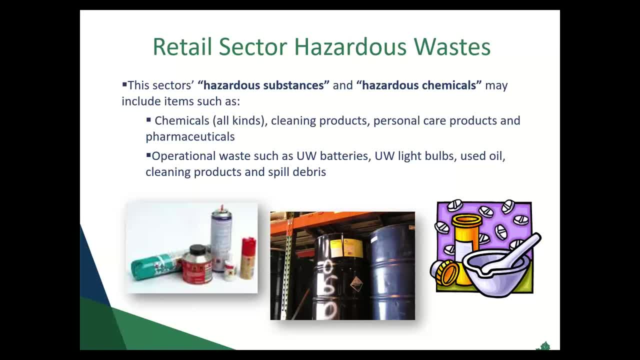 for the um, hazardous weights or types of hazardous weights that are generated, and chemicals. it's a kind of laundry list, depending upon what kind of you know if you've got a, if you're a pool supply company, a pet store- um, yeah, everybody's got cleaning products or personal care products. 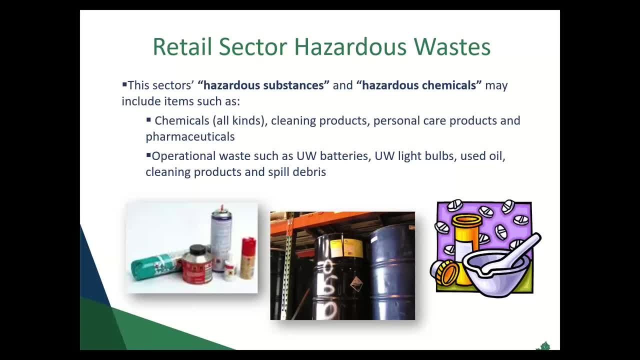 you know, like some of the, the, the perfumes, uh, some of the hair products, uh, and again the pharmaceuticals- and I think I throw in what I would call the operational waste- you know, actually run in a building or if you have a distribution center, what are things that you know you could? 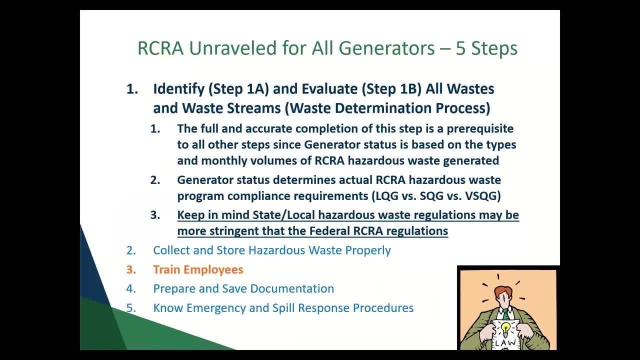 you generate there that have to be factored in right, getting more towards the uh, um, the, what I would call the. this is sort of my five-step program, uh, to trying to unravel um hazardous waste, and I think I've used this before, but I I bought a book called 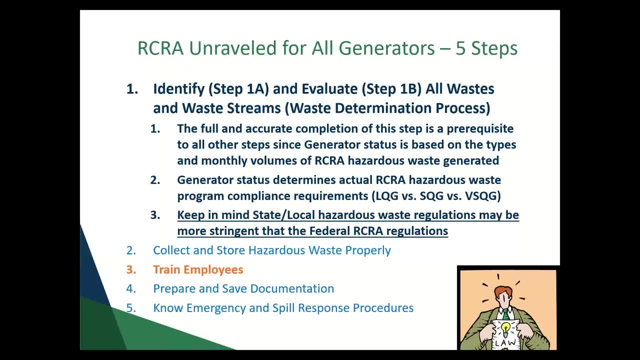 um, it's almost like a record for dummies, um, and you know, and it's, I think it's like 1200 pages. whoa, yeah, because it goes into some interpretation. sorry, dummies won't read that. I know I've actually been clicking them, but I mean I speaking for all the dummies out there, yeah, well, I've brought that. 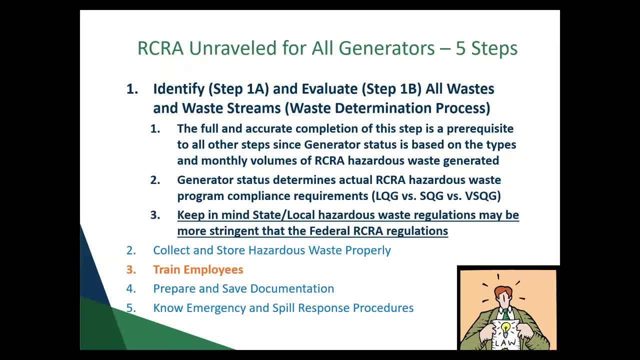 to some training sessions, sometimes when they, if someone or an organization asked me to do rekra training for 30 minutes, so I bring. okay, here's the record for dummies. that's 1,600 pages. where do you want me to start? yeah, uh, and what we're covering today is just a tiny part of this, and 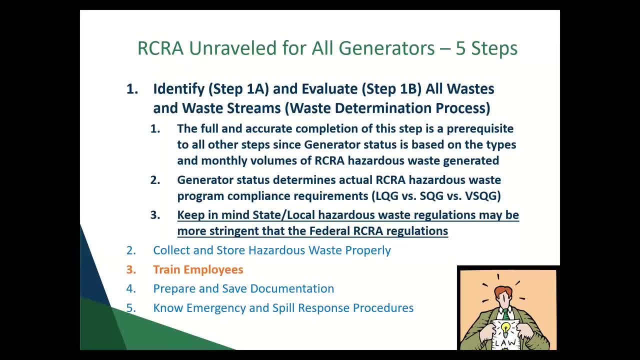 I again. I part of it I said earlier is I want to focus on sort of part uh, identifying and evaluating the waste, because I think that's really is the primer for all theelVEHXcom of this and i call it step 1a and 1b essentially is identifying what waste you have and then going. 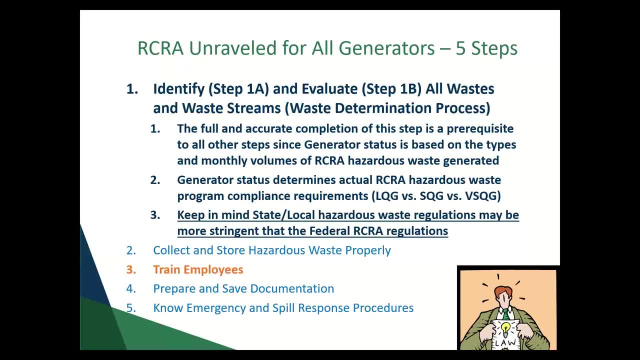 through an evaluation, or what we call a waste determination process, so that you know which of those wastes are recra and which are not. and then, so that is sort of the step one, and that's a prerequisite to all the other steps. um, by doing this step two, you you then have an ability to 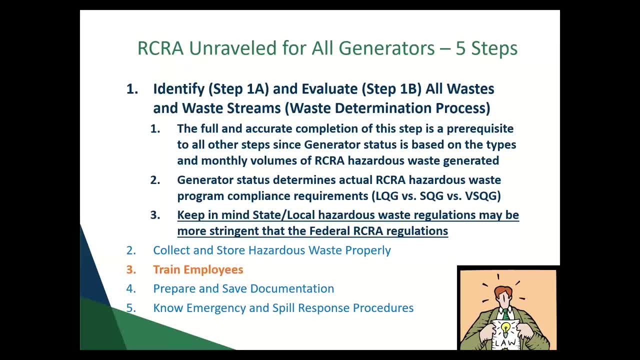 understand or guesstimate your volume of each of these on a monthly basis, which then you determines your generator status. you know large, small versus very small, um so, and what i'll cover here in a second is sort of the federal you know game plan, and you have to don't discount what the states. 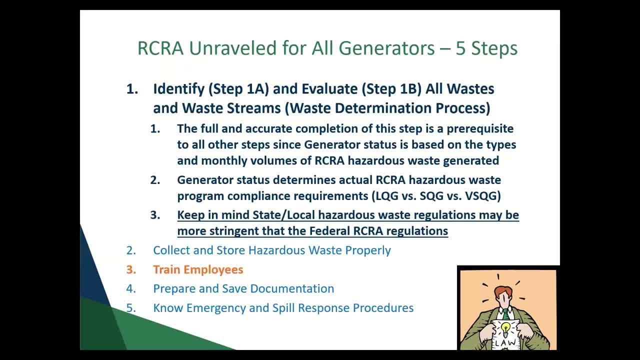 have, because i mentioned earlier about minnesota. um, maybe, maybe we were talking about it, but a waste from a retail pharmacy in texas, uh, would be non-regulated recra. that waste could be hazardous waste in minnesota because their rules are different and minnesota has more strict rules. 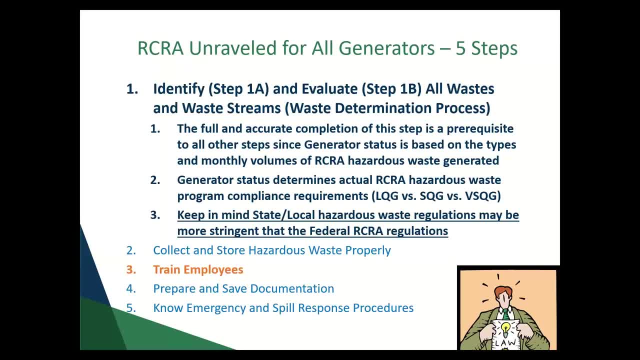 than texas. interesting. so same same exact grains, different, okay, different standards, okay and regulations. and then there's once you know what your your, you identified your waste and you've gone through in the waste determination process and you've at least taken a best shot at what your generator status is. then you do the rest of these. 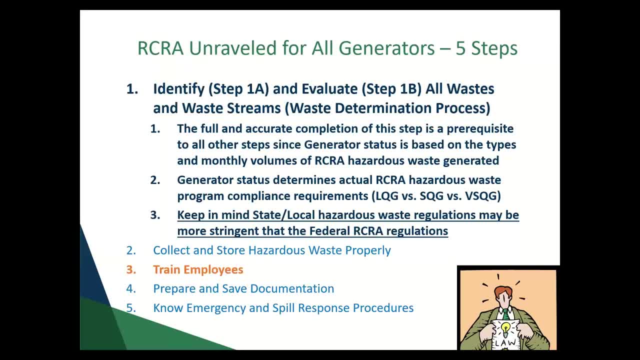 like two, three, four and five: collect and store, train employees, uh, and i'll cover a little bit more on training because i think that's i wanted to do that. and then there's documentation, inspections and then spill response. things like that are part of the program. so this is sort of a 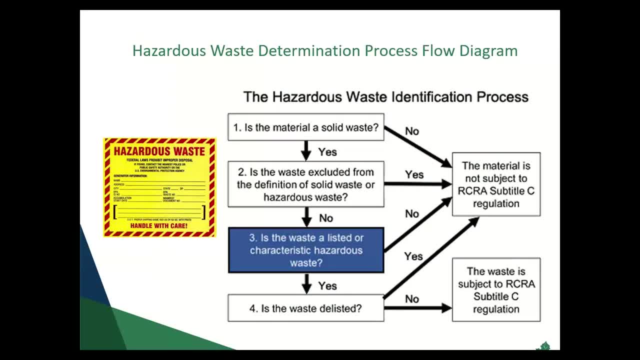 quick uh, next slide: waste determination process flow diagram is: and again, this is the federal sort of a, the. the general process is, you know, you kind of go through this chart, uh listed waste versus characteristic, um, and if you know, and we could have, literally we could go and for days just. 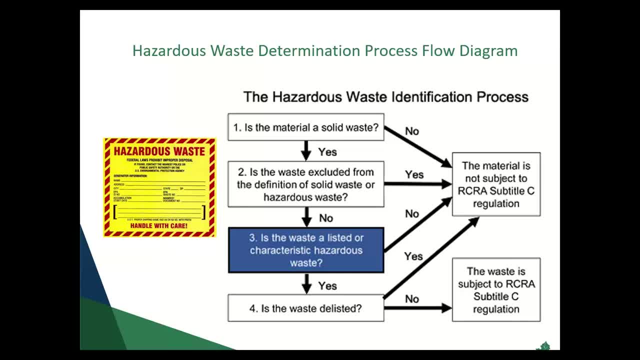 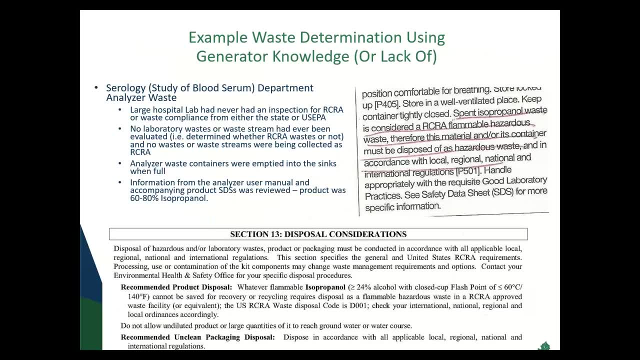 talking about listed versus characteristic and how to figure that out, um, but this is sort of the the menu and the flow diagram of doing this for each of your ways. in the next one i think i used this last year. i kind of modified it a little bit, but, um, one of the ways of 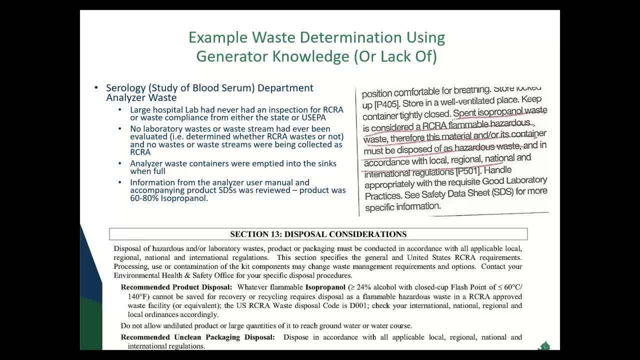 a waste. determination of your waste is generator knowledge, and generator knowledge is the individuals who are working with that waste, or chemical right, And let's just use this as an example. So this is an example from a department, a real department, at a large hospital lab that I 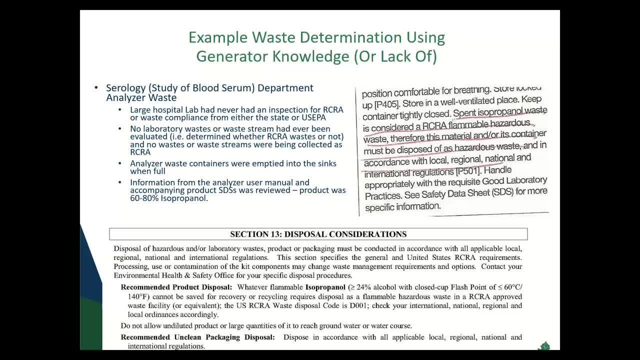 was in and kind of some background. They had never had an inspection for RCRA or waste compliance by either the state or the US EPA, ever. They had never generated hazardous lab waste. This particular analyzer: it does a blood serum analytical. 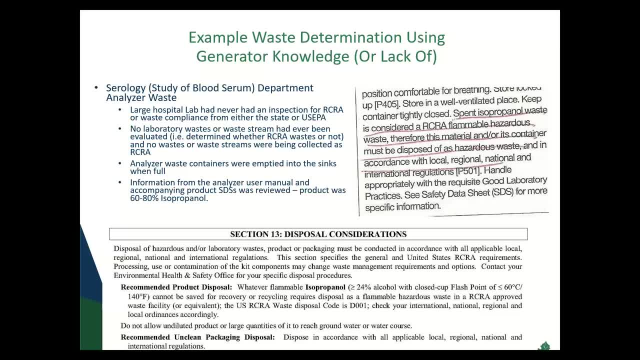 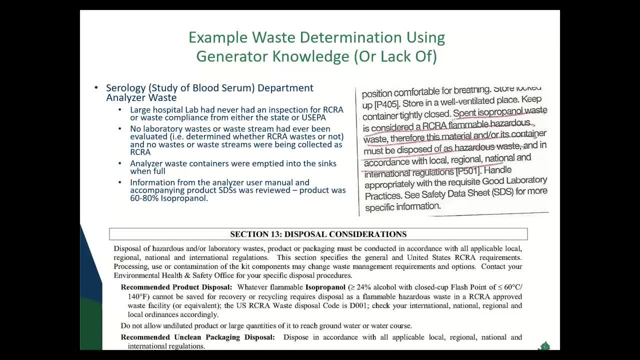 And the cleaner waste falls into a what I call a jug or a plastic container underneath the machine. And so I walked up to the machine, I opened up the cabinet and I asked the technician: what do you do with this waste? You know, because it said, it said a waste bucket. It was, I remember. 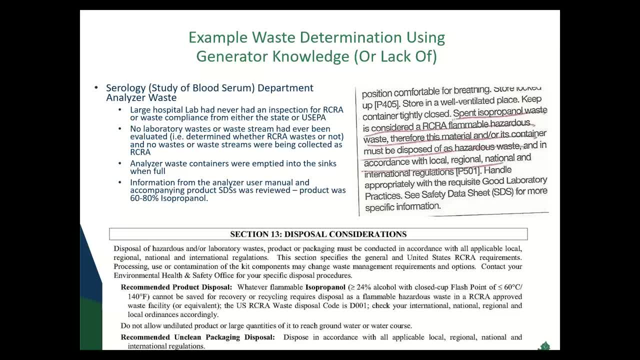 and I asked what waste goes in there, She said, well, that's the from the. I thought the shear guy, That's the waste from the cleaner. Okay, When- and they said when it fills up, we walk over to the sink and pour it down the sink and 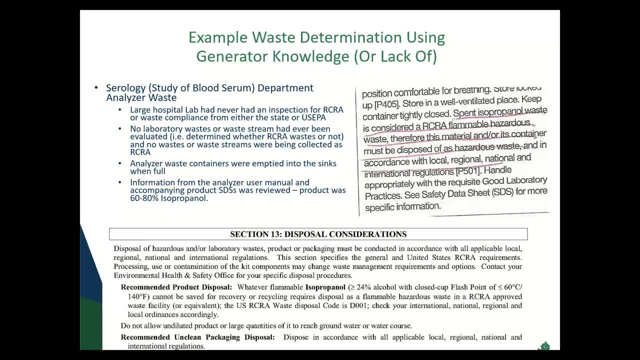 we put the container. Yeah, So I start scratching my head and going, well, do you know what's in the cleaner? You know? no, no answer, no response. I said so then I start thinking to myself: do you have a operations manual for the book or, you know, for the machine? 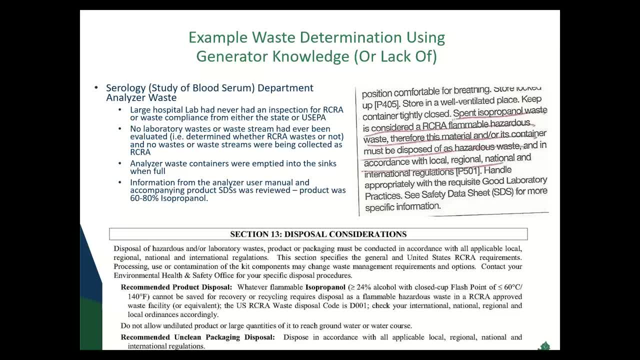 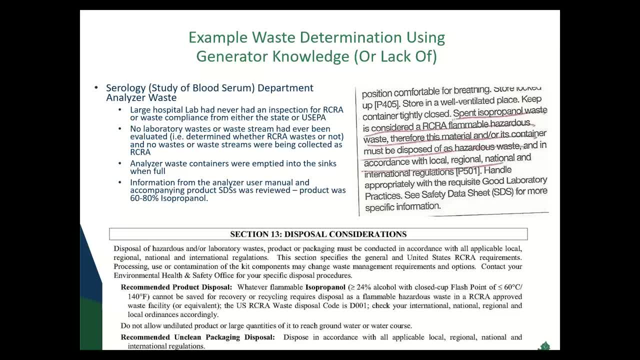 Yeah, And I took a picture- that's the upper right-hand corner there, a picture of a, the disposal section or part of the disposal section, And it says, I underline, I said spent isopropanol waste is considered a record flammable, hazardous waste. Therefore, 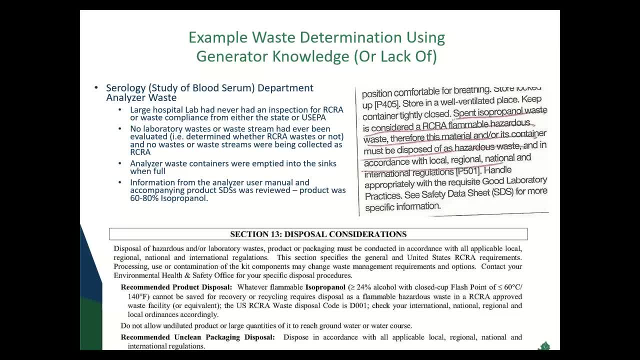 this material needs to be collected as okay. And I said next thing: I think, well, it's a product. They buy this product, this cleaner. Do you have a safety data sheet on it? Oh yeah, We have that. Speaker 2. And then we dug that out and I snapped: 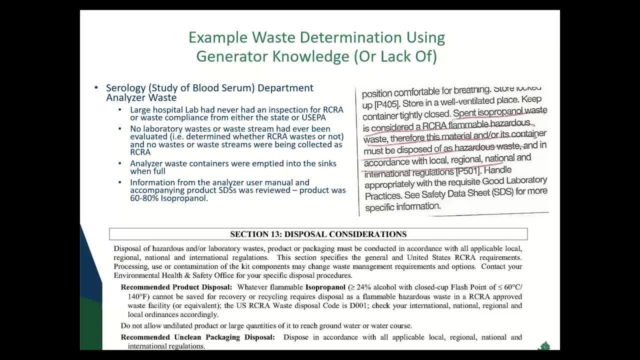 the section 13, which is disposal considerations for this isopropyl cleaner, isopropanol cleaner- and if you know it's kind of small there, i did it, you know i blew up as large as i could. uh, it's flammable, hazardous waste. d001 needs to be managed that way. well, and i'm with the safety. 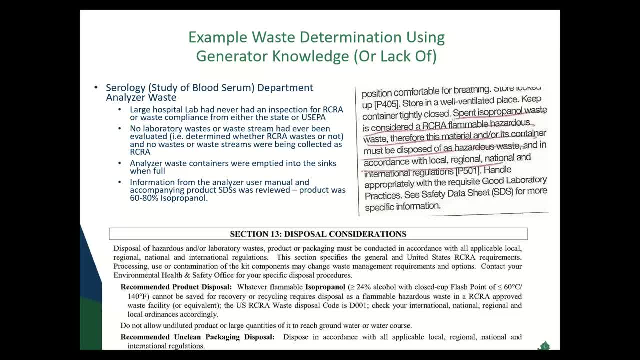 director of the whole system. i'm with the lab managers, i'm with the facility manager, i'm with the technicians and they're feeling like really bad. you know, i'm not trying to put anybody under the bus, but this is this is a pretty easy one. um, it says right in their own operations how to deal. 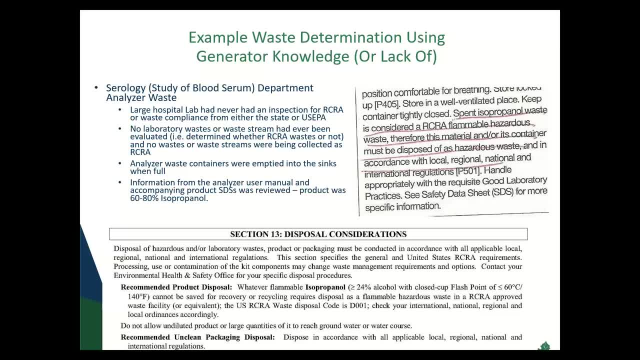 with this but in essence, since, primarily because no one had ever asked them, they were just doing the thing that they've always done, uh, it in. in essence, and from the moral of the story, this is really easy to collect. it's not that hard to manage, right, it isn't going to break the bank. 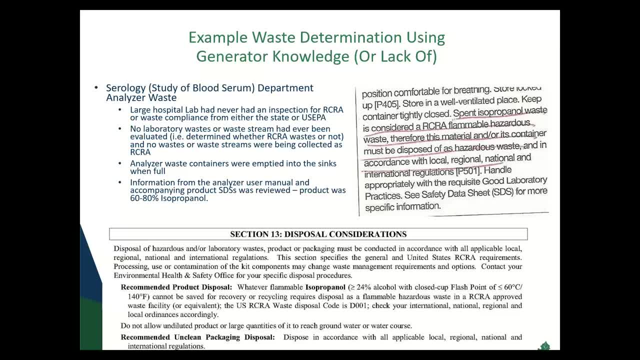 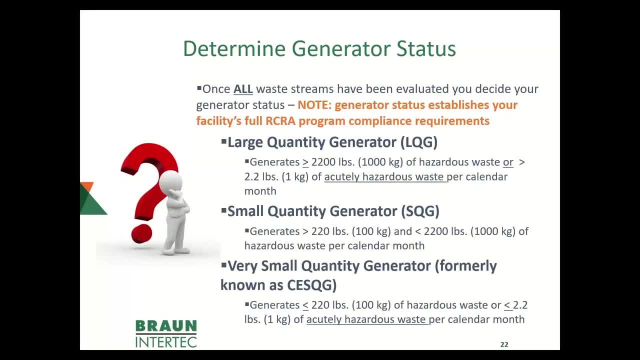 in terms of cost, but it is the proper way of collecting and managing this waste and if you get caught and they decide to fine you, then that could be right. very much so once a individual or a generator goes through that process of, you know, identifying their waste. 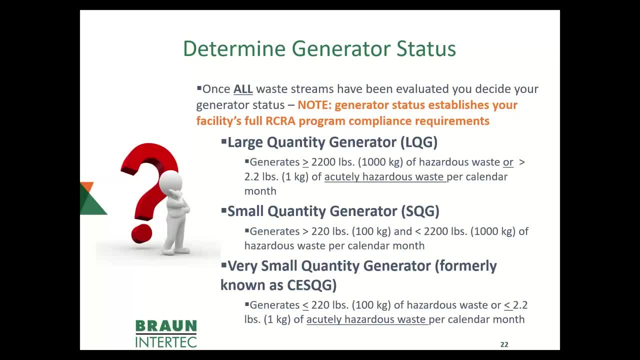 and then determining, uh, the volume and which ones. in doing that waste determination process, then you've got to figure out your generator status. so this is really a key to knowing what your compliance requirements are. um, because if you fall into the large quantity, you have the most. 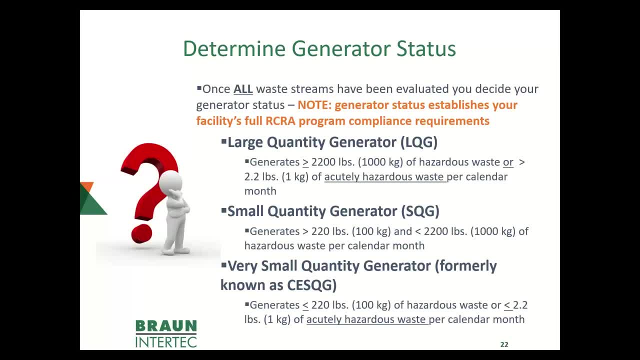 compliance requirements, and small quantity is the middle and kind of the very small, which is the new word, and then you've got to figure out what your compliance requirements are and then you've got to figure out what your compliance requirements are from the federal- you know- changes. some states still use the cesqg kind of acronym because they haven't adopted the. 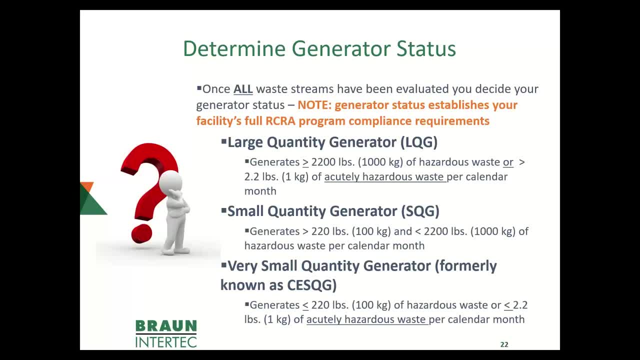 the generator rules yet. so, um, not all these are exactly the same in some states. some states have more strict definitions of what's a large quantity generator, so you have to sort of know that too. but this is the federal list, all right, i said i kind of cover a little bit on recra training, um. 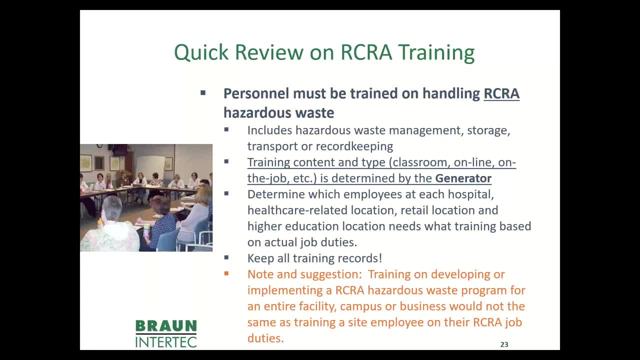 and so there are- um, there's no sort of set recra training. in fact, the federal regulations on training are kind of uh, they're not very prescriptive on what it actually means and why. i think they did that. is they really kind of forced the generator to figure this out themselves, like who needs what training and why? 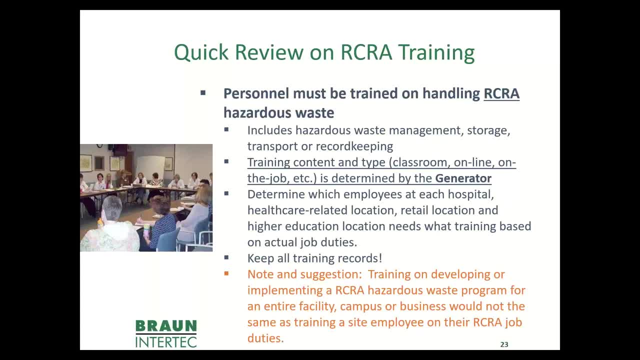 and sort of that's because of the bottom. here is: um, if you were building a new facility, like i said, and um, and you know you have, you know you're going to have waste, how would you design the program? what i you know, i would probably train the management of. 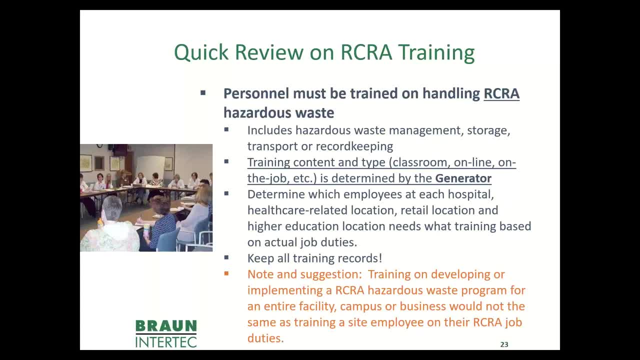 that facility on what is all of recra right management level, and then, how does it apply to our building? what do we do first? we do, okay. identify waste, do waste determinations, uh, figure out generator status, find containers, store them right, you know. train employees. what well, we train. 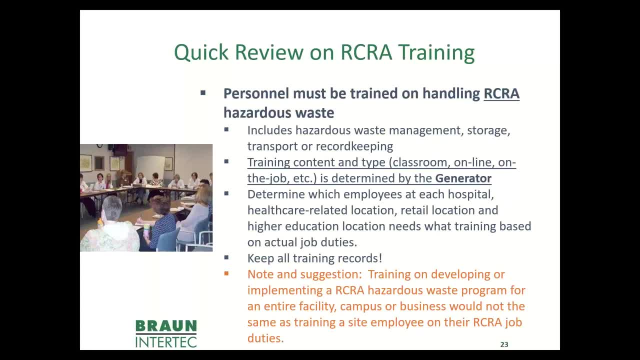 employees on their job duties. um, so the kind of the easiest thing to think about is, in turn, like a hospital, like a nursing right. it nursing can be as simple as what is hazardous pharmaceutical waste and what container does it go into? yeah, because that could save you a lot of money. because if 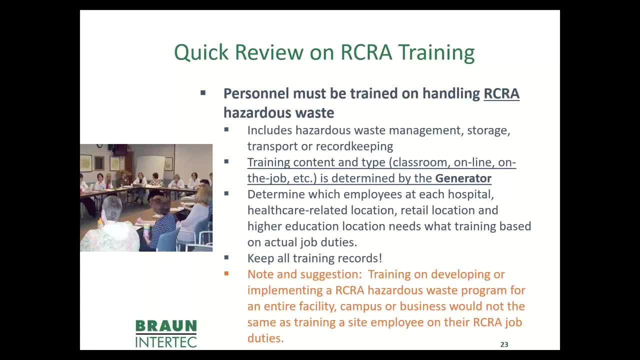 you're putting non-hazardous waste in, like if you just don't know, and you're putting it in. yeah, i mean i'm not even getting into that. yeah, so i mean that could just to save money part would be be great. i'm always thinking about that part. yeah, it reminds me of um. 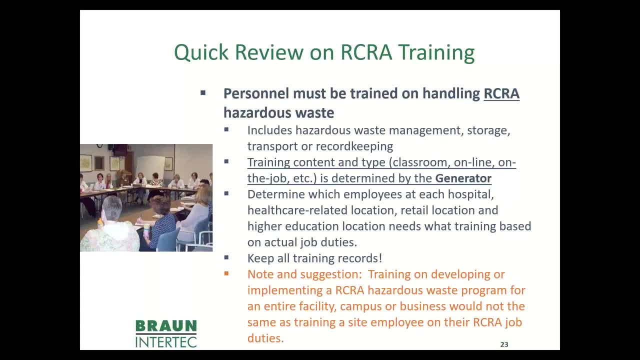 where i was earlier this week out in new england state um, the pharmacist was indicating to me of looking like going and doing their own little self audits of their containers- hazardous pharmaceutical waste containers, uh, and they're finding lots of stuff in there that doesn't need. 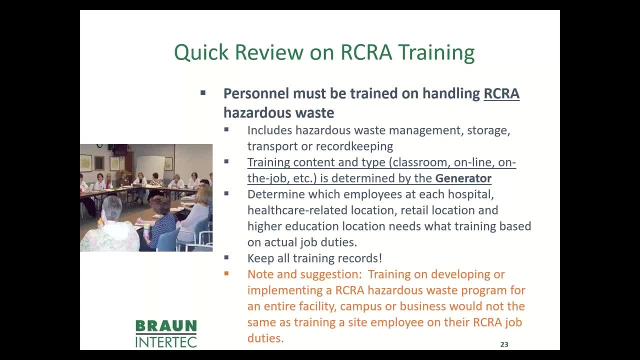 to be in right and that's yeah and it's so. it's just compounding it and if, and part of it is they in, no, no, no offense to what they did, but they kind of created their own way of of doing something, but they didn't really think about how to do the training to the actual 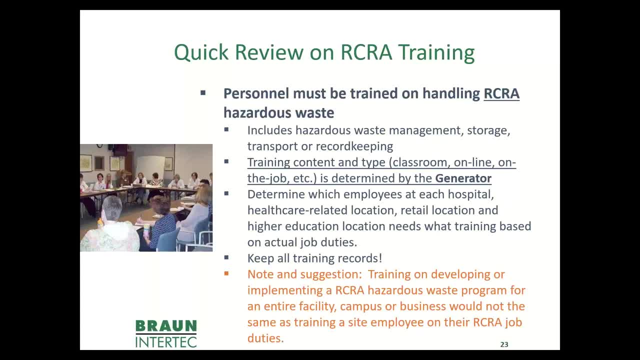 generators of you know the nurses if you don't know, if you have somebody you don't know, i don't know if this is hazardous or not. it's better safe than sorry. well, i mean, that's probably what, yeah, but but better safe than sorry was good for the odd thing, right for the standard stuff you know. 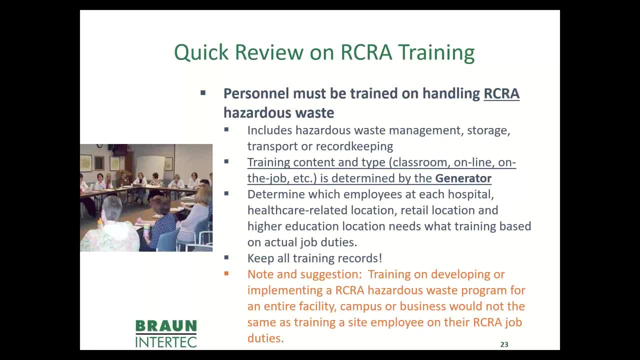 we don't want to be collecting non-recra, absolutely hazardous waste in record containers, right? um? so this is really a key thing. is that, uh, i, i, kind of i, i, i, i disconnect what i call program or sort of strategy development implementation level training for a team or a leadership versus the employee training of a staff. 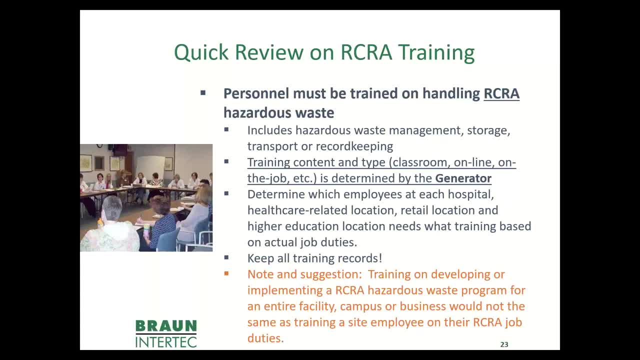 with duties. right, if the staff duties is. i move a hazardous waste container from point a to point b. that's all i do. i know what's in it. that's my training. i do not need to know how to do any reports. i don't have to do. i will wait until next week to know how to do any reports. i don't have to. 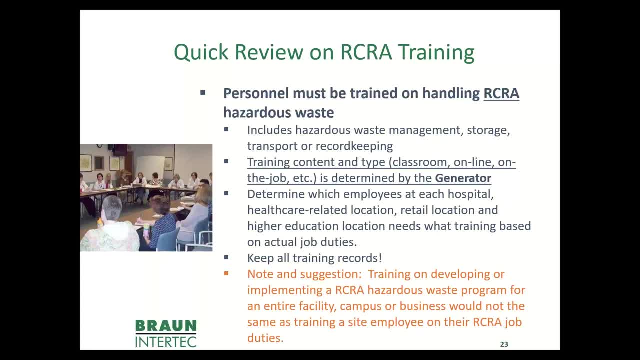 know how to do any reports. i don't have to know how to do any reports, i don't have to. you know, i don't really care about my generator status, because that's someone else is dealing with that. so it's really a function of what is the person's job right and, and that's it's really i. i can. 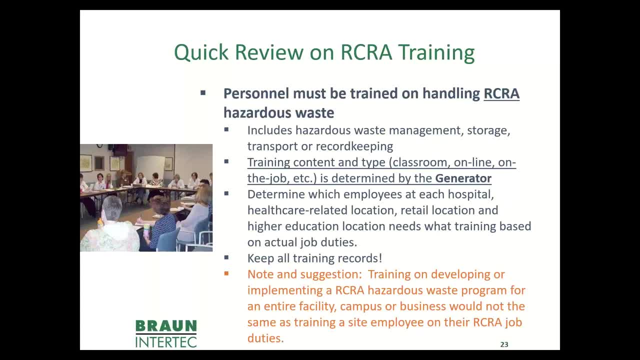 this probably is complicated in the retail world as well, because you know, um, pick a store like, uh, so everybody's going to be dealing with some kind of, some kind of hazardous material. i mean, it's just the way of you know, way of it is, but you just have to know. 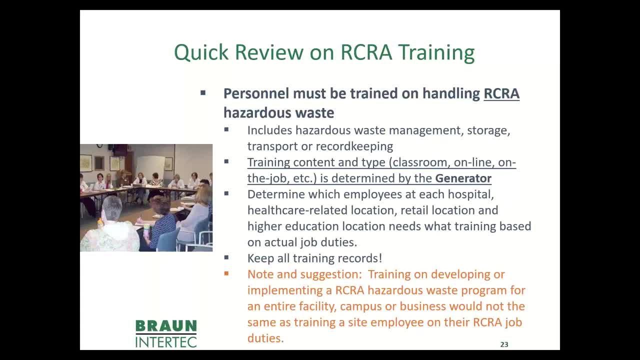 how to, how to, and many times there's an online version and i know some of the waste companies have you know. you can do subscriptions or you can do online portals to do that. so i'm gonna, i'm gonna do a shameless plug here. so this we, most of our listeners, probably know. 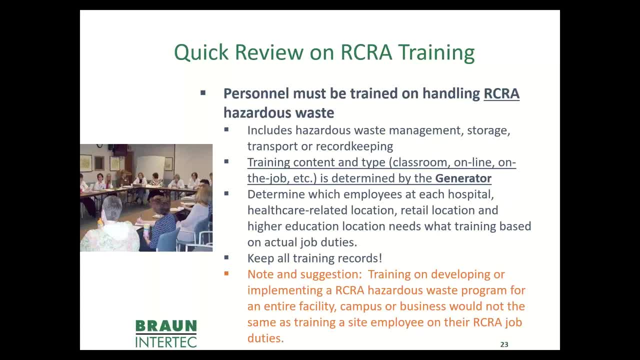 that we always offer a record management training, um, and we do it, usually do it in three different cities: dallas, houston and then, uh, san antonio and austin. um, but this year we're gonna do it all because of covet, we're doing it online and we're doing it, and so it's going to be. 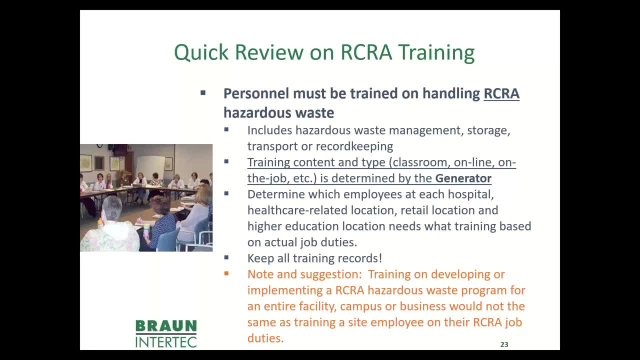 a little bit different than what we did in october, and if, um, i'm going to have lydia actually, uh, put that on the letter of the email that we send out to you guys. so you look at, i mean we're talking, it's 75 and if you know that, i mean that's an amazing price and this is for people. 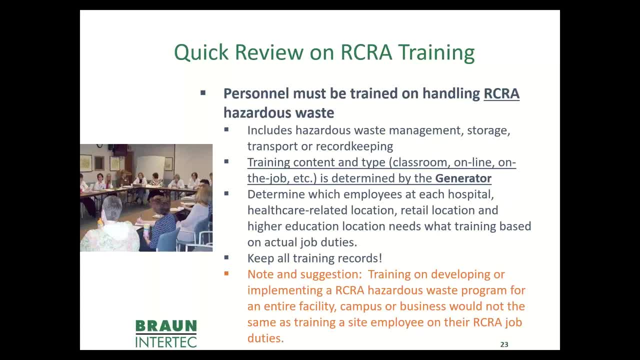 that have already kind of gone through record training. this is because they're a refresher and you have to do it every once a year because that so, but uh, it's um, yeah, so that'll go into a much more detail on all these topics. yeah, and so it's an. it's a lot of work, but it's a lot of work. 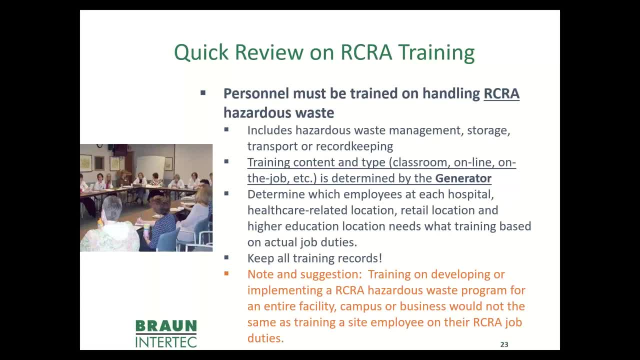 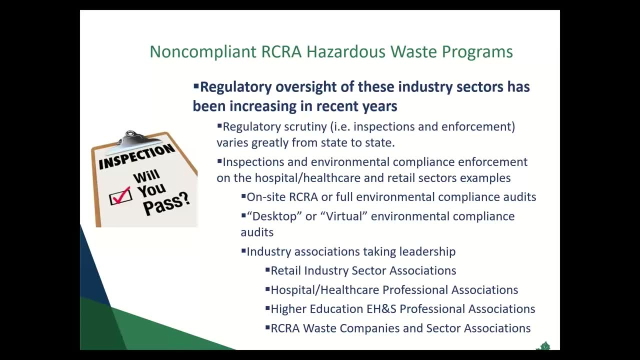 an eight hour course and so, but, uh, for, for the price? um, because it's usually we usually do it for, like you know, 399. so, but so there's my shameless plug. there you go. sorry, i had to throw it in there, all right, uh, this, and we're getting close to the wrap-up, um, sort of what it would be. 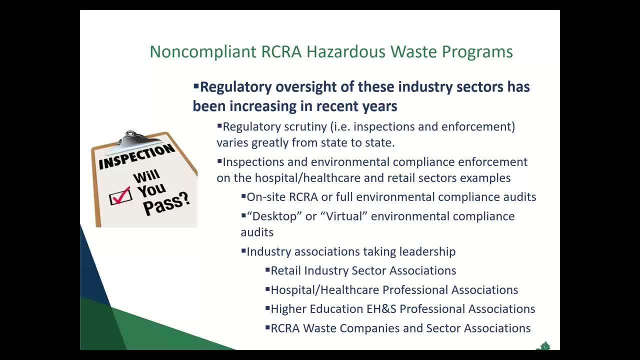 a non-compliant, you know, hazardous- waste program. well, there in, in general, regulatory oversight for these particular sectors has been increasing. um, you know, i've seen it in the hospital space, for sure, and then in the retail, yes, and then in the retail space, for sure, and then in the retail, yes. 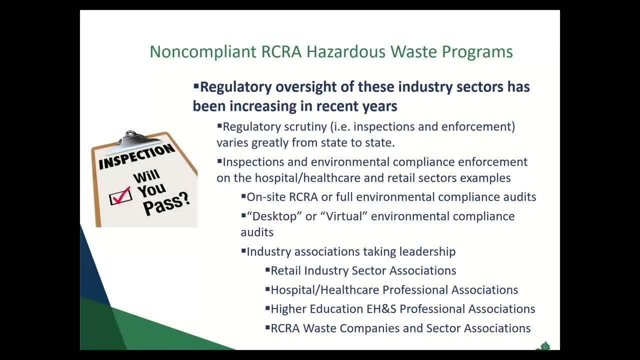 i mean, there's been some large settlements and other things that are, you know, are easy to find. um so it you know what is happening for the regulatory scrutiny that really varies from state to state. so you know a and i'm kind of go back to the hospital world, the 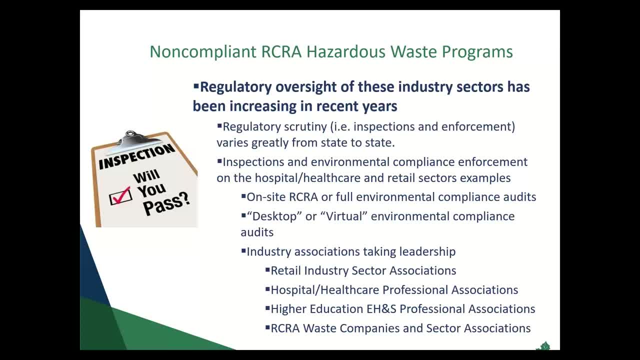 this the one where they had the lab waste. had never seen an inspector of any kind ever for hazardous waste. um in minneapolis, st paul, where i live, the county go to every hospital every year, so you can imagine their programs for hazardous waste are way more fine-tuned and 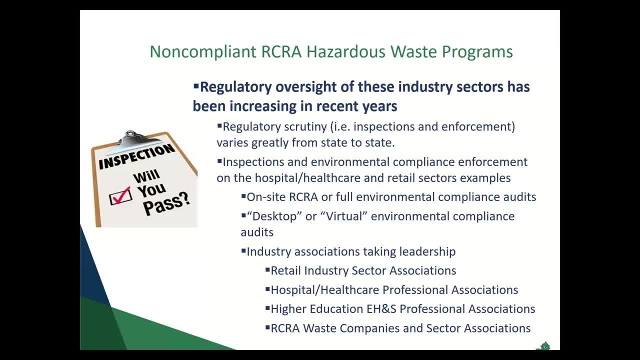 no upsets, uh, hardly any kind of violations. you know an odd thing here and there, but pretty much runs on its own and people know what they're doing. uh, if you go to a state that has never had anybody there, you know you, you never know what you're gonna find, um, so inspections can be, you know. 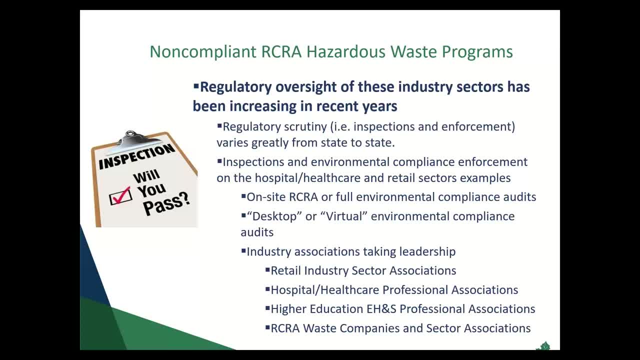 If you know about the environmental auditing world, you know there can be RECRA, hazardous waste inspections. there could be full environmental compliance like Clean Air Act and stormwater, and you know EPCRA and all these other. you know federal regulations. 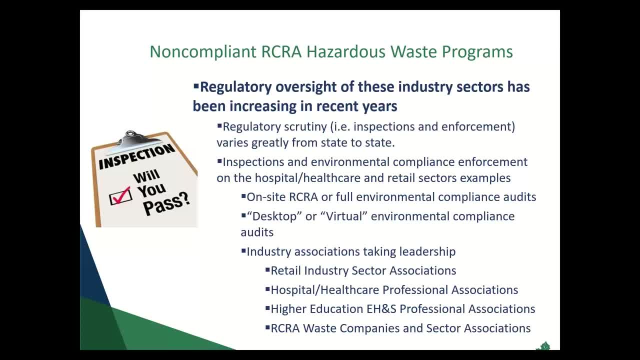 We're going to talk a little bit later about desktop and virtual, which I think are pretty common right now, And what I've also seen in these particular industries- you know these industries we're talking about- is the associations are taking some leadership. 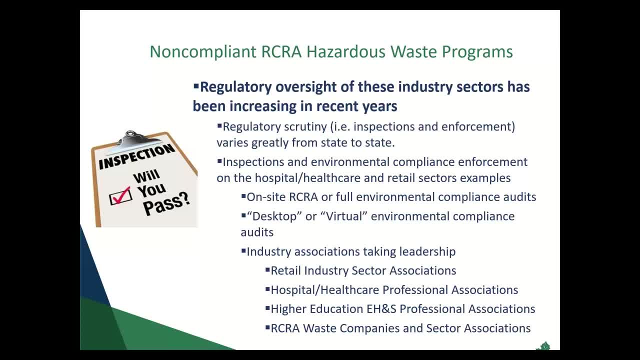 In fact, I often go to what's RELA? RELA is the Retail Industry Leaders Association, and it's an association that supports that industry And a lot of the big retailers are part of that, And there's excellent information on their website in terms of compliance information, hazardous waste, you know, status of various regulations and things. 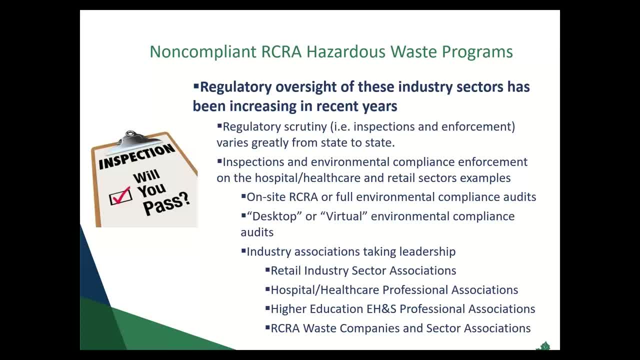 So that industries are picking up the pieces here In the hospital and healthcare world. there's the professional associations. I'm a part of a couple of them: The physicality, The physicality engineering side, and the housekeeping and EVS side. 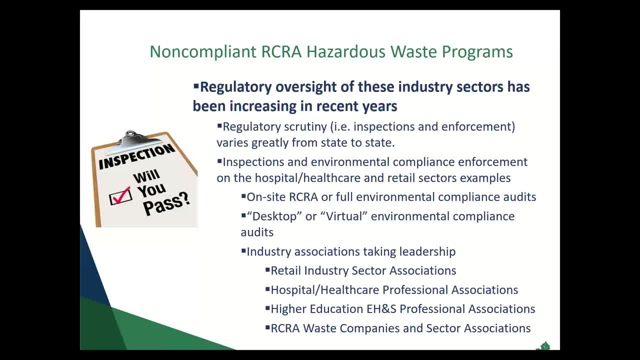 Higher ed has. one is called the Campus Safety, Health and Environmental Management Association, which is basically an association of professionals, EH&S, professionals that work in higher education, And we mentioned some of that. you know, we know some people in that world. 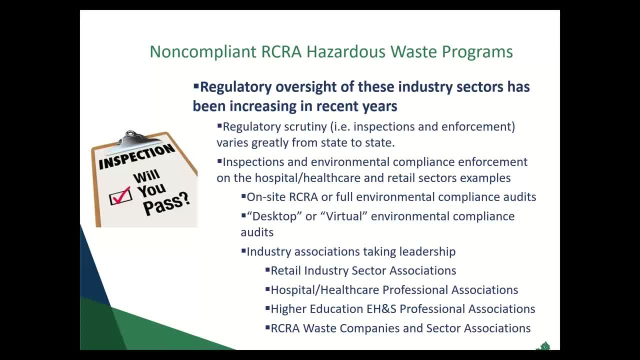 The other. the last thing is not last but least, but the actual companies that service the vendors that are picking up waste- And their associations are pretty- are very active in this. you know doing webinars or updating, you know taking leadership and trying to help understand this. 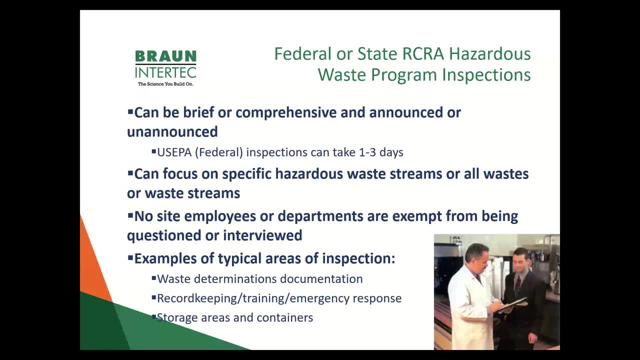 This is pretty. you know, this is pretty common. You know, if you have inspections, can they be brief and unannounced. comprehensive, Yes, any or all of those things, In fact. I'll tell you about one in a second here. 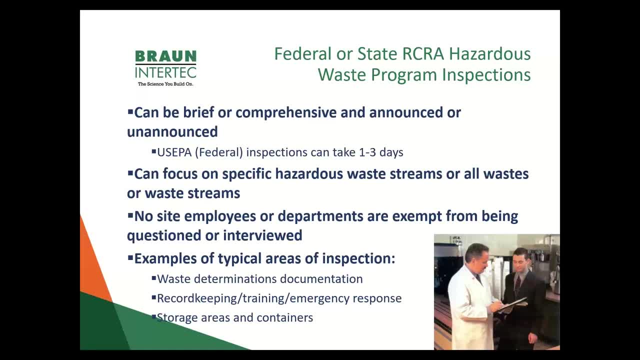 So when I'm working out in New England State Was an announced virtual inspection. So the hospital leadership got a email from the state inspector saying we are doing what we would call a comprehensive environmental audit of your facility. We are not coming on site. 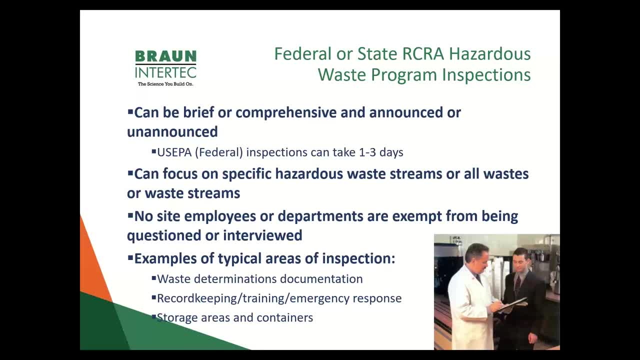 Here's a three pages of bullet points of information we would like you to gather and send to us. The clock starts today, And that's where I was last Monday, Tuesday, my head spinning. Was that an emergency? Hey, Darryl, get to Boston, or were you already scheduled there? 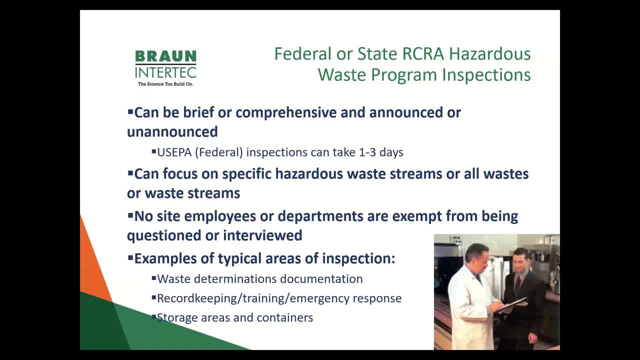 No, this was a separate. Ah, okay, Yeah, it's been. it is what it is. Yeah, You know we're doing what we can and helping where we can, But ultimately they have to submit information. If it's there, it's there. 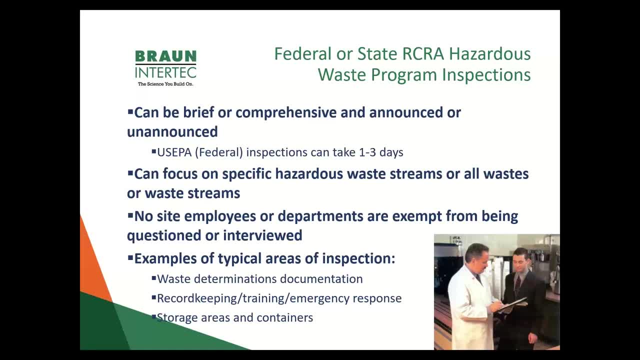 It's not. it's not. And then again, at any kind of facility, the employees or any department can be asked anything. So that particular Particular request of information covered a lot of stuff. I mean there is underground storage tank. 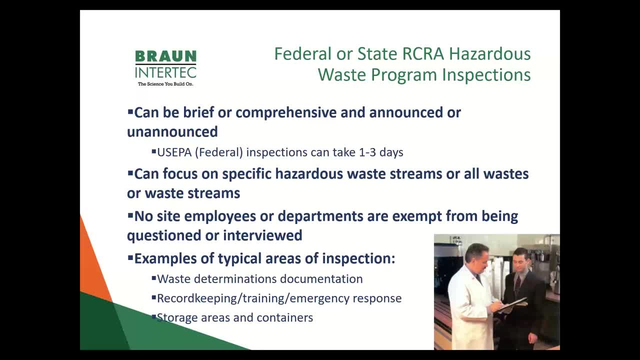 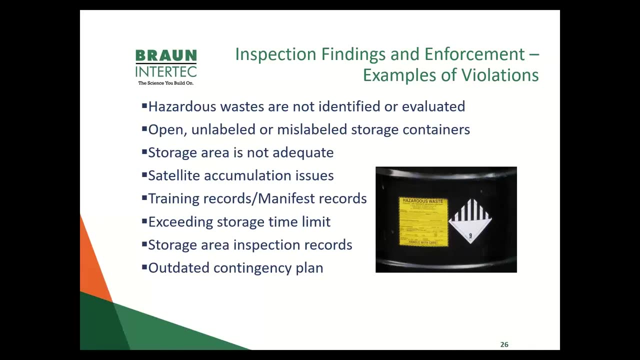 There was boilers and Clean Air Act information. There was hazardous waste, universal waste, training records, DOT training. You know it was pretty comprehensive. Wow, The next one in. people have seen this before. This is sort of this is what inspectors look for: training records. 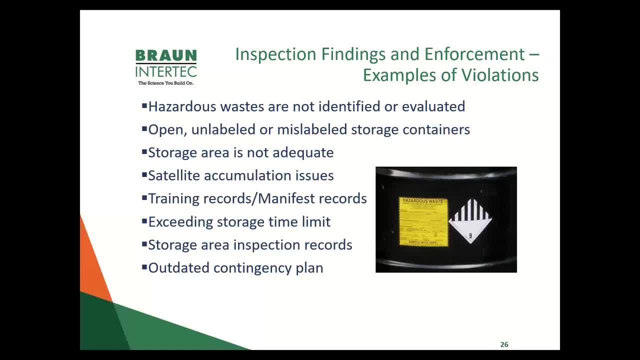 You know they asked for training records for the various departments at this facility. You know, did they do inspections of their storage rooms, All that kind of stuff. So this is common kind of violations and that information dump, which I'm going to call it to the agency, is going to be large. 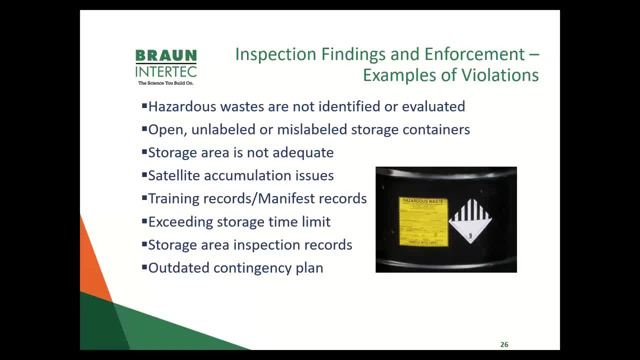 And I'd hate to be the agent trying to go through that, but there's someone's going to do it. So at the end here sort of more like program management solutions, what I see when I think of an executive team is sort of the management of the building or the management of the company or region and what they think about in terms of, you know, risk management from a regulatory standpoint. 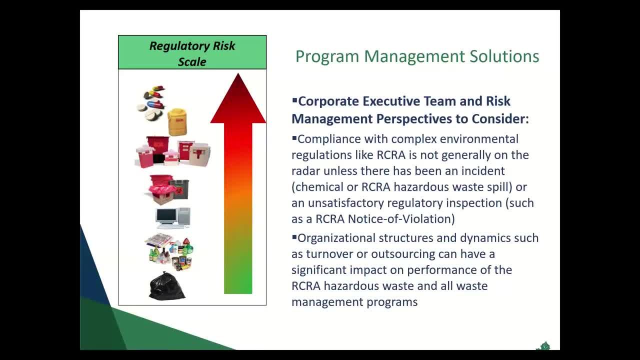 And this I've got to go to the next one, I'm sorry. The scale on the left is sort of like: as you get higher into like pharmaceuticals and solvents and kind of the higher risk wastes, your requirements are increasing, your costs are more, your training things are more. 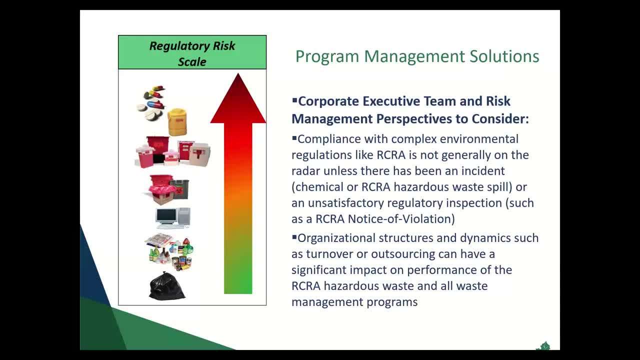 So this, this is sort of a scale of you know, everybody has trash, right. It's, it's easy, pretty easy to manage the ultimately as a business And as an agency or someone that I'm inspecting that facility is you want to put things in the right container for the right reasons, right? 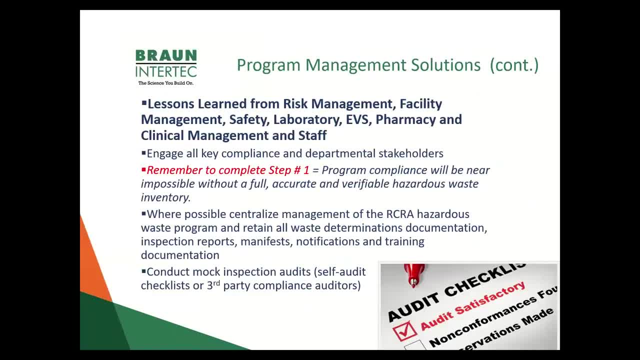 And you keep working on this, Let's go on to the next one. So then, from a what I call lessons learned, from kind of department level, folks within hospitals and within educational institutions and perhaps, to some degree, retailers. they're not going to have all these departments. 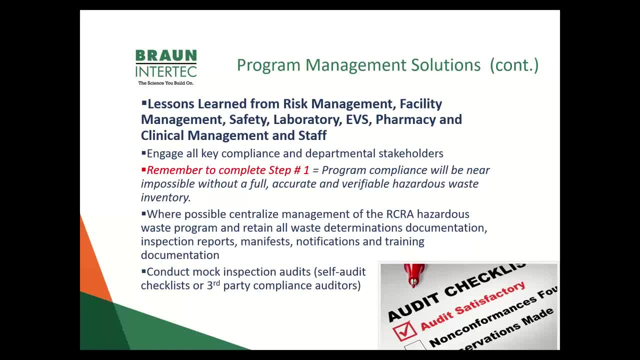 But you know, as you're developing a program and you know about the compliance, you really Need to bring in all the pieces. Part of the working with this hospital is going through this inspection- virtual inspection out in New England- was the lab had done, I mean pretty sophisticated and robust. 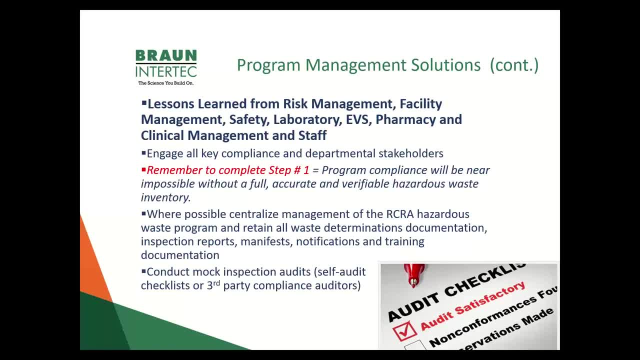 Program for managing the lab waste, but they didn't really incorporate what was happening in pharmacy or facilities or used oil or all the other parts, and so it missed out on things. They're really sharp on that one part because they knew their. They're really sharp on that one part because they knew their. 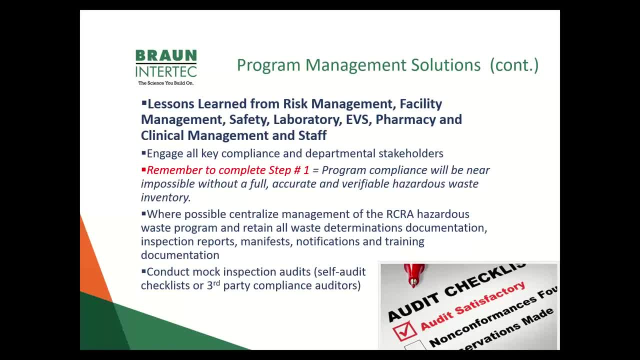 But as a individual that runs that facility, You're going to think about it as a building. You know you can't just have one department doing their own thing and the rest of it's ignored, because the agency is looking at the building, Right. 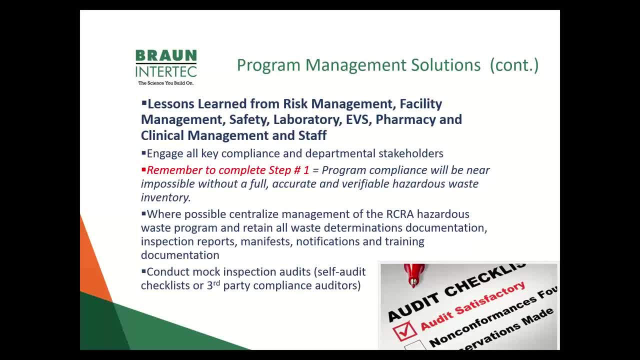 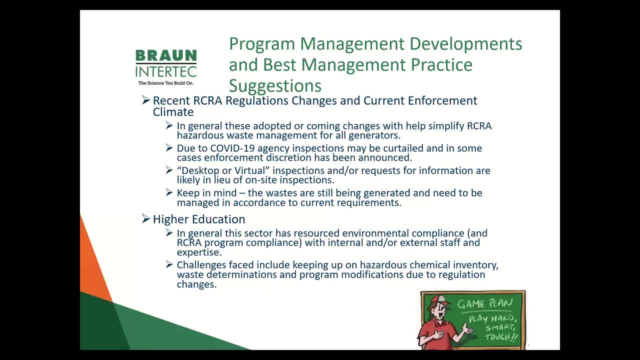 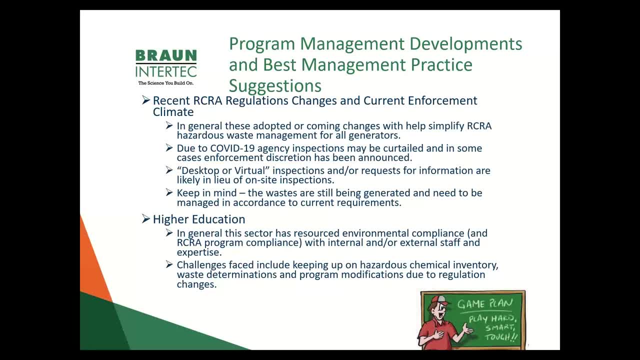 You know. pick the states that are more You know. pick the states that are more, states that are more aggressive or more enforcement scrutiny. or pick states that have like regulations you know. or look and also look at like the waste streams that are really more risk to your. 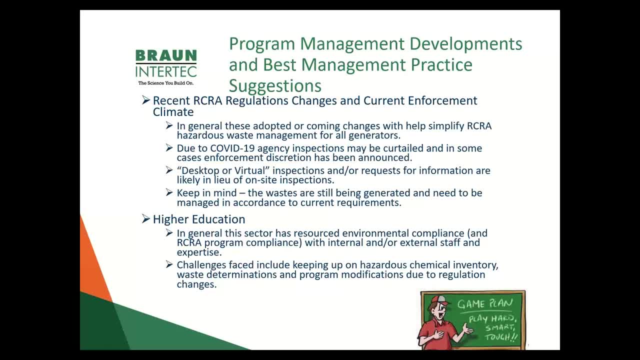 employees and compliance and you know if there's a failure like a spill, what would be the worst case scenario, and then kind of the last year, is: how do you do any kind of like internal auditing? do you do checklists or do you do audits? do you? i mean, i've done- i don't even know how many environmental 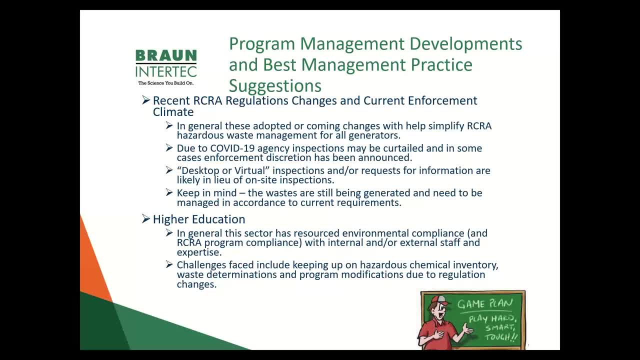 audits in my life. um, so you know, working in factories and refineries and chemical plants, going in and doing a true environmental audit. i'm there for four days. uh, it doesn't happen. in some of these you wouldn't need to be four days at a hospital. so uh, kind of at the end here on 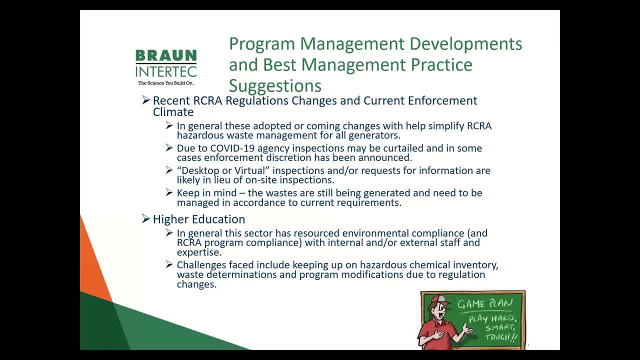 program management and some suggestions. we talked about the recent regulation changes in general. all those changes that are adopting are coming are are going to help simplify hazardous waste management for all generators, so that's a good thing. um, we mentioned a little bit about the agencies and, due to covid, 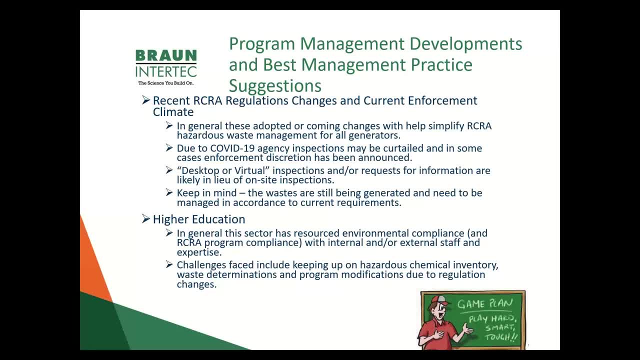 from their ability to do enforcement, uh, or inspections, uh. i think there's going to be more. they will, you know, they're not going to go on site. they're going to send a request for information saying we are essentially doing an audit of you. here's what we're going to need to look at, and 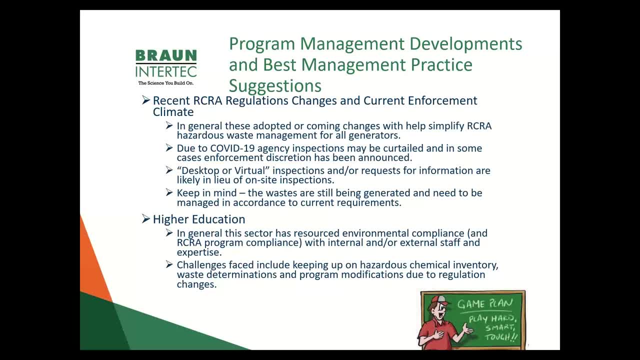 then here's a time period for you to generate that information for us, and they, they literally did have a time frame. i think it was like a two and a half weeks, maybe 12 days or something. wow, um, and then kind of at the you know, no matter what else else is happening in the world, whether 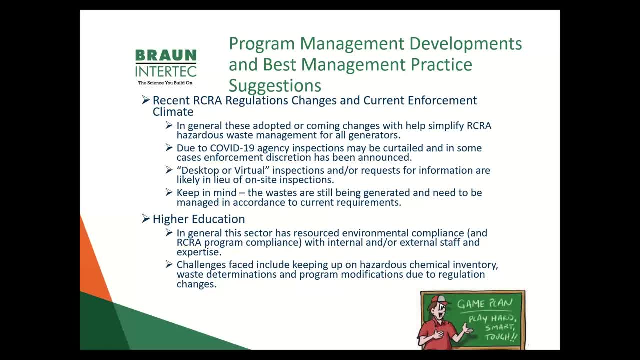 it's, you know, infection or elections or whatever. the waste is still there, they're still being generated and you have to sort of know what your need to comply with. and so when i break out like higher education i- i think it's just more of a observation because i've worked a little bit in- 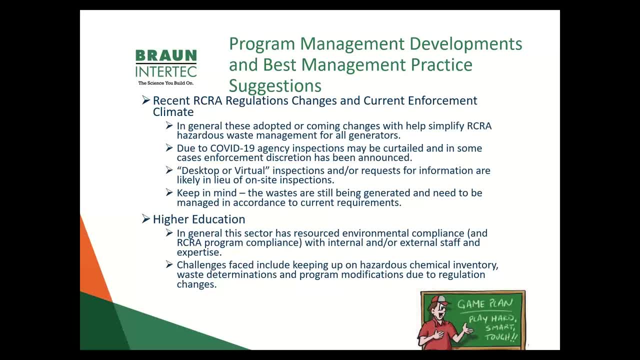 that, not as much as i've worked in the health care or the other industries, but they essentially have some good internal and external information and i think it's going to be a good time for us to external resources and staff. they sort of got you know they. they know who, what they do and they. 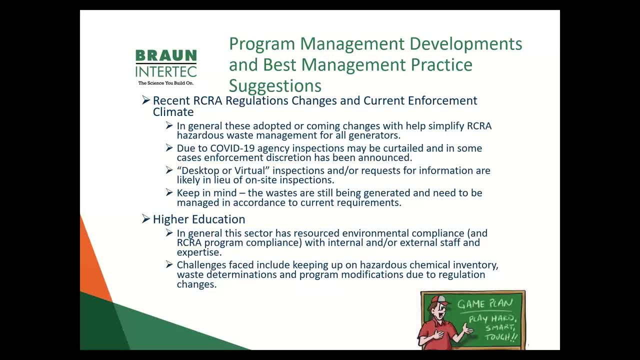 they have some ability to manage it themselves internally with some skills and some uh individuals, so they kind of staff it the right way. uh, they still have challenges and obviously keeping up with chemicals like what is new chemicals coming on the building, waste determinations, and then with these regulation changes, how do we modify what we're doing so that we 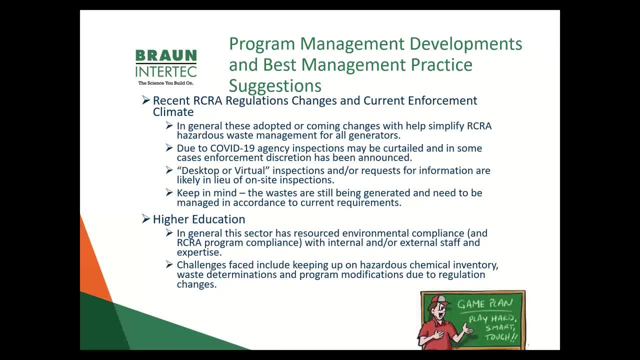 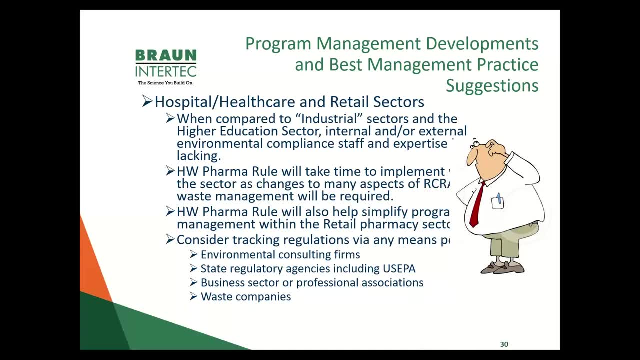 yeah, modify to to take advantage of the and kind of the last one here is the hospital and health care and retail sector. i sort of lump them together because, relatively, compared to the industrial sectors or even higher ed, the expertise in terms of environmental staff is is is lacking. i mean, in some cases it's got. 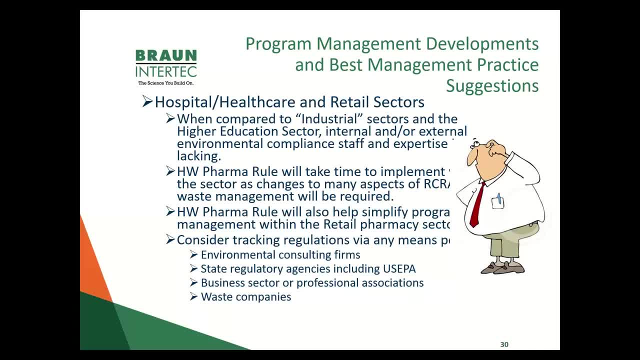 some there, or it's changes a lot, or most of the time i see it's worn by the. the environmental hat is broken into 10 chunks. it's worn by 15 people, so no one is really in charge of the whole thing. the pharma rule is going to take some time to implement, because if you just choose to just 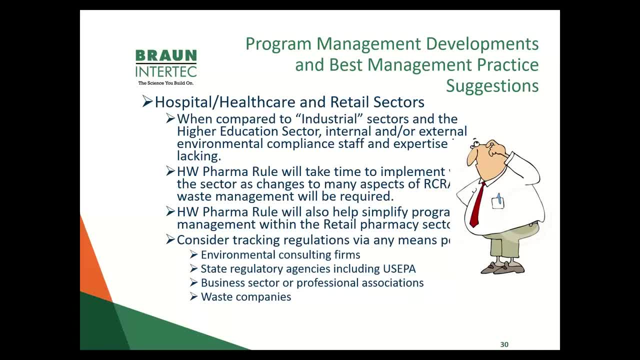 we're going to set up our program according to that. you have to make changes on how you're managing the pharmaceutical waste. now to do that, which you have to maybe retrain, get different containers could be reporting differences, but in general, if you can do that, that's a good thing to 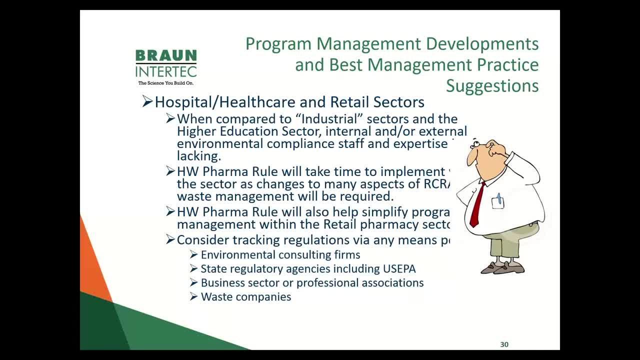 do that, and it also applies to the retail pharmacy sector. so, lastly, kind of what would you? how would? i think the biggest thing is tracking where your relations and what they mean. and again, i would go to the. you know people like us that have environmental, you know, consulting. 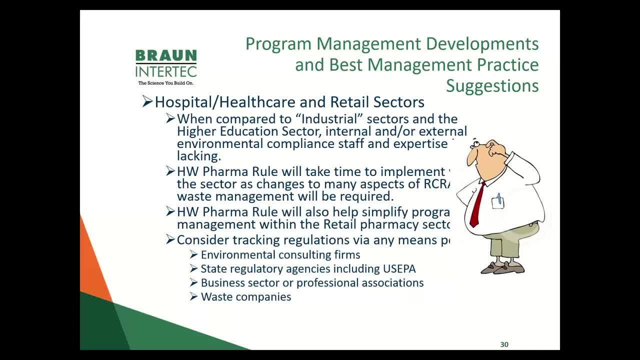 skills. i mean we do this for remediation, for investigations, auditing, compliance, environmental health and safety. you know ocia, we, we have that. we know what's going on in the states that we work with. um, then you go to the agencies, including the epa, and i've given some 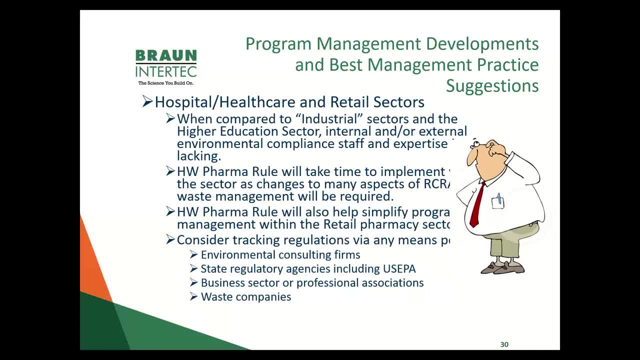 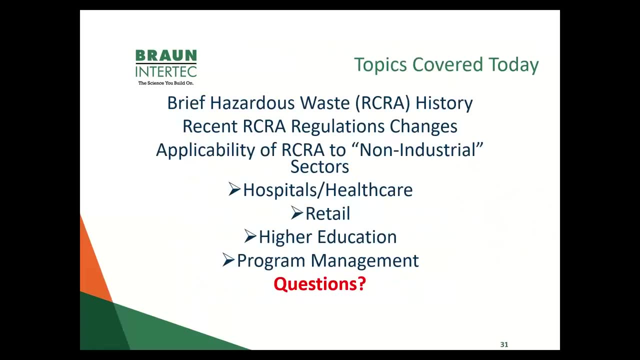 links on there. and then i would also tie in the business sector and the professional associates that I'm a part of. some there are really good ones and they cover parts of this, and even even the waste companies do a lot to help their customers. yeah, cuz they've seen it before and it's easier to this worked. we had this similar. 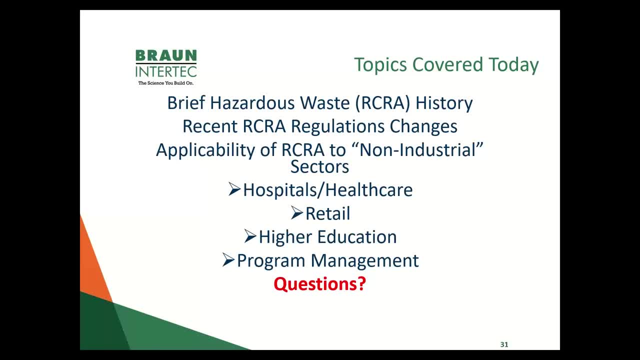 situation in this company and we can do it here and yeah, so we're kind of at the end, Lance and I. wow, that was fast. yeah, I'm dry, but these are the kind of the main topics we covered and and we can drill into any of these in more detail. 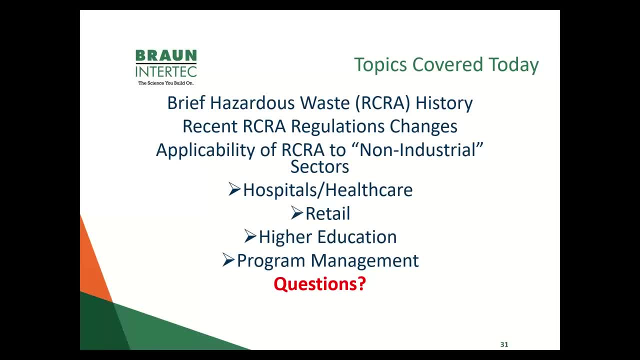 but it's, it's. it's an interesting area to work in regulations to keep you on your toes, yeah, and and and. then you have you know again either the announced or unannounced inspections that happen, and and it's kind of like a fire, fire drill. 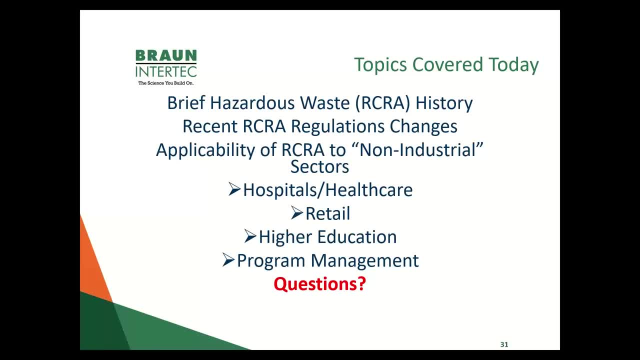 to get the paperwork together. and again I've seen there's probably- and I told the people out in New England- there's things that they're going through. I've seen somewhere else and it's just a matter, and now we got to get our arms around it and work through. 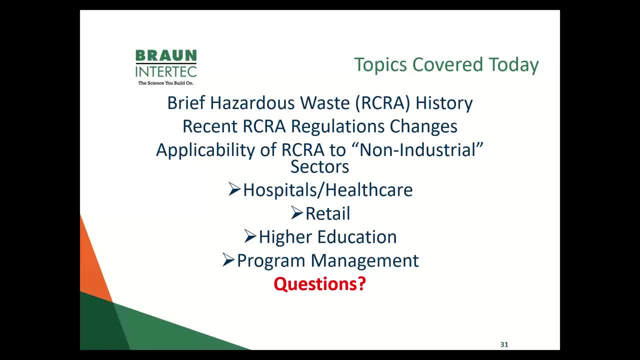 the process to get them up. yeah, and, and, and there's, in looking at some of the regulations being sitting in on the record classes, there's a lot of. there's a things change with the littlest and or, but. you know, and or butts and you got to. 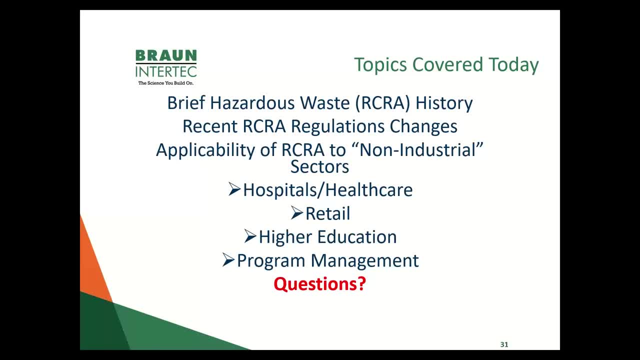 really make sure you watch those because it's you know you got to kind of pay attention so it can change. even you know, in that that paragraph it can be interpreted different meanings. so we are running a little short on time, uh. so I do have there's a few questions, but I'm 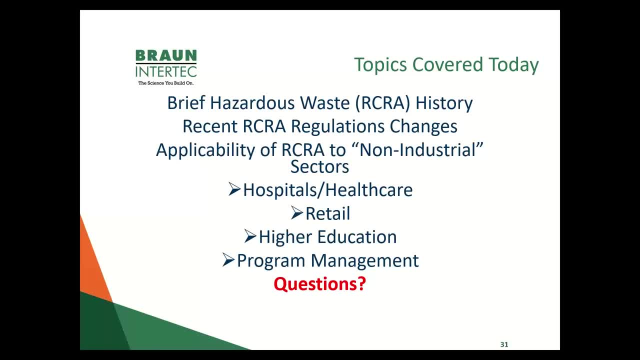 going to make sure that Daryl gets them in. in response, uh to to you guys. but I didn't want to clarify. one thing is on the record: training that we were doing, it is going to be several states, not it's not just going to be one state. 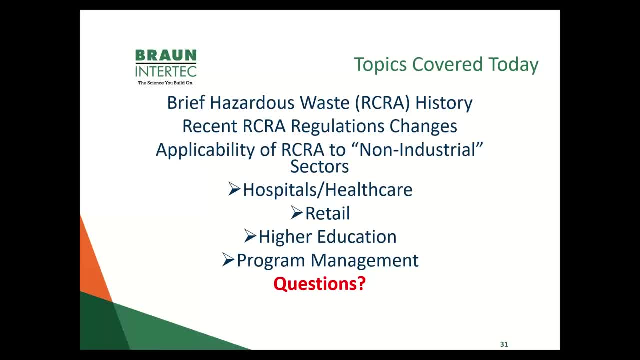 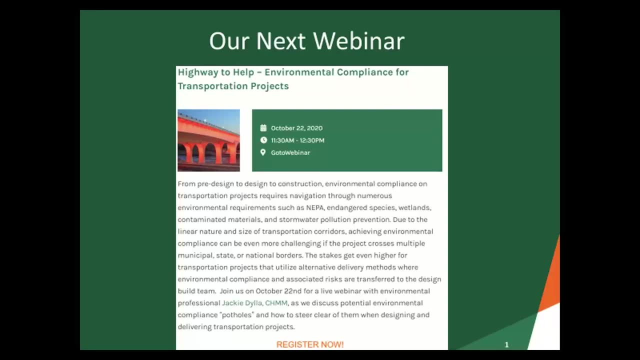 specific, so we are going to generalize it, so it's so. don't worry that if you're like, hey, because normally we it's been Texas, but now we're going to do them all nine, 11 states. so, uh, I just wanted to clarify that as well. our next webinar is, uh, on October. 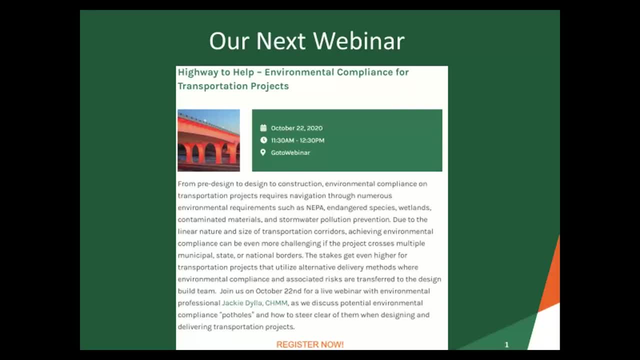 22nd. it's um going to be the highway to help environmental compliance for transportation projects. you gotta sign up for this webinar. just for the fact that they haven't AC, they reference an ACDC song, so we're really excited for that one. uh, Jackie, dial is going to be, uh, our expert on that.